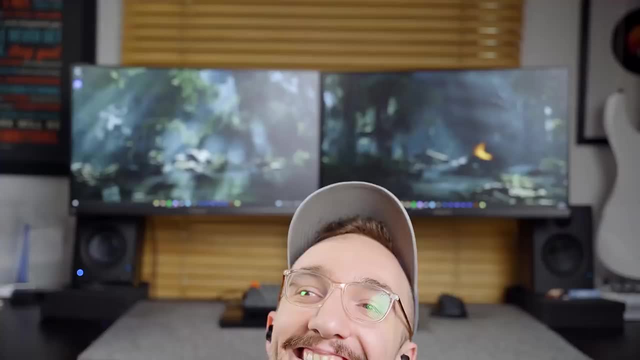 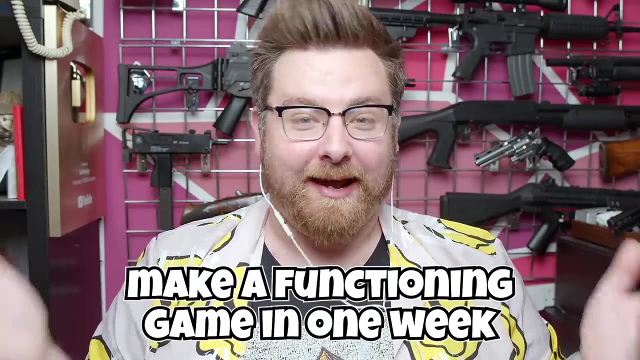 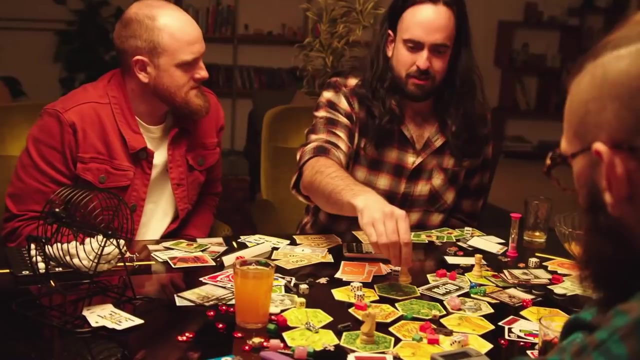 I am on the floor. Oh no, Elliot Goff and Eddie Bowley, and also me. You have one week to make a functioning game. Um, Okay, It could be a video game, a card game, a board game. 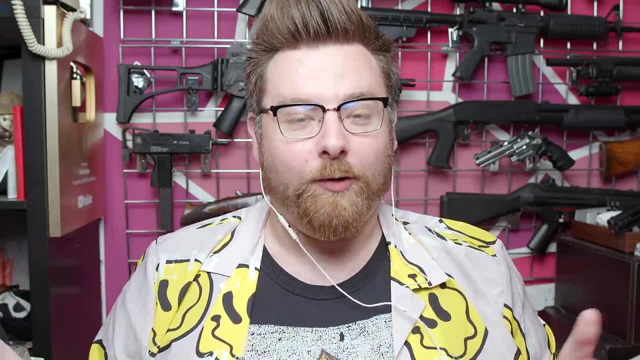 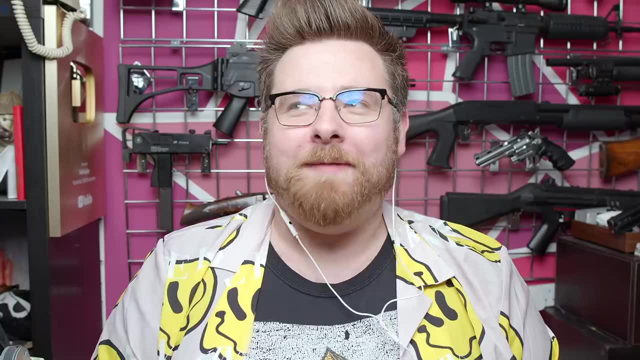 It could be any type of game, but all it has to be is ready for the three of us to play in a week. Is there a win parameter or is it just We played the game and the best game? Maybe the win condition for this episode is who actually wins the games that we play. 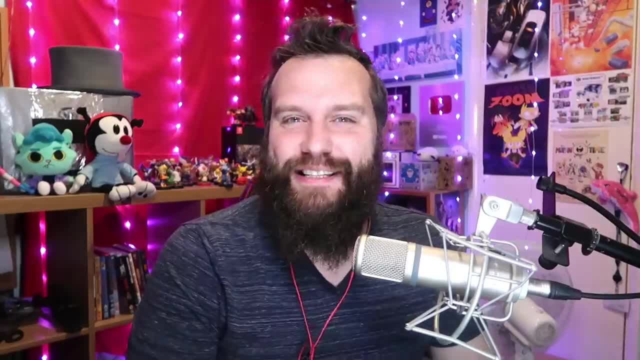 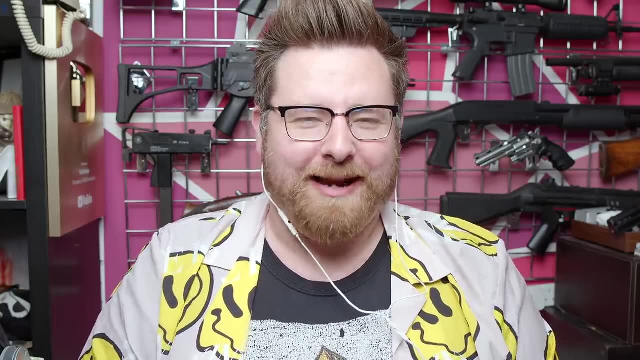 Oh god, okay, We can just rig it in your favour, so badly. We can each rig it in our favour, so badly. That is the. you know. Elliot could make a game called. Is Your Name Elliot? You win. Are you ready, kids? 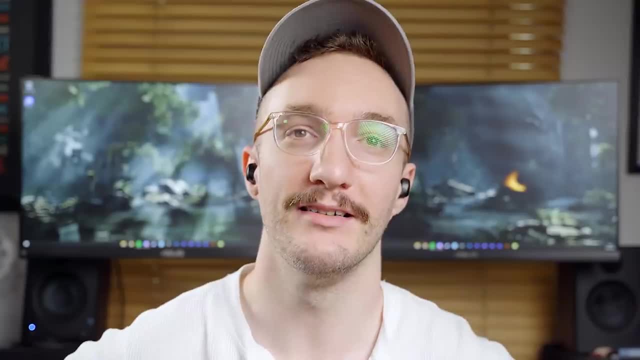 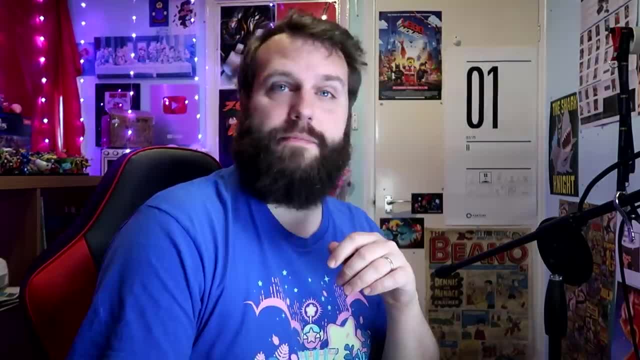 Okay, so make it a game. Okay, so make it a game. I guess I'll go with video game. Let's make a game. Christ, okay, Oh, my god, Oh god, okay, It's actually teaching me the game. 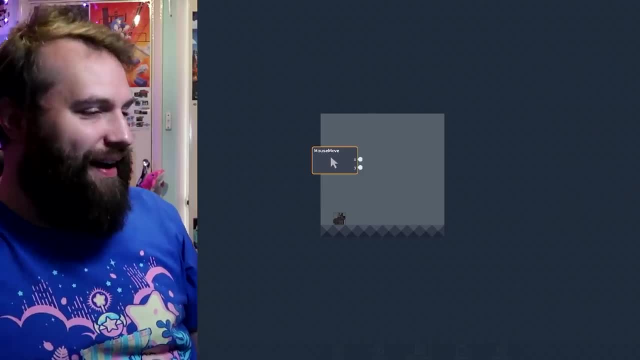 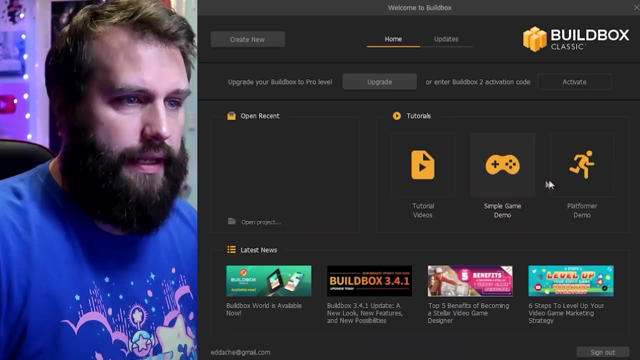 I want a man. I got a dog. How is this simple? Fuck, I can't move the doggie. The fuck do I do? I wanna like move the cursor around and it moves the doggie around. I just wanna move the doggie. 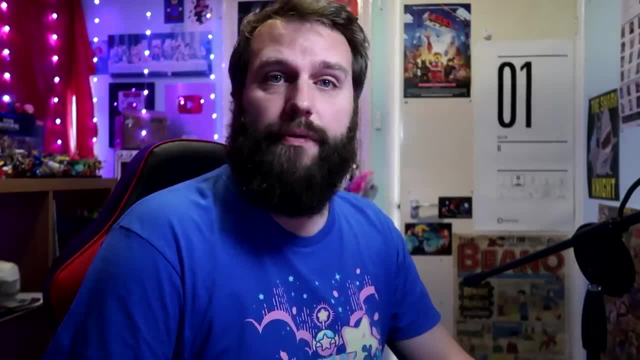 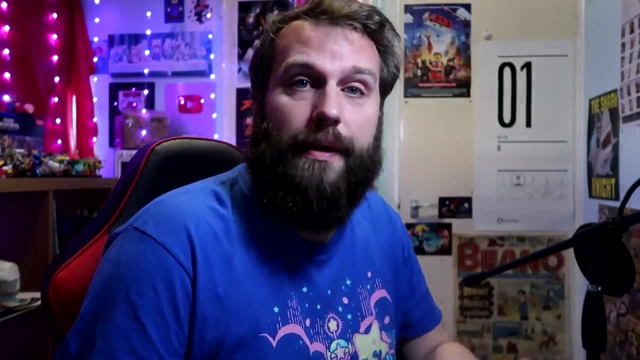 Let's try a simple game demo, Because I'm a simple game boy, I'm a ball Christ. Oh no, I moved the wolf. I moved the wolf back. I really just wanted like a drag-and-drop kind of game maker. 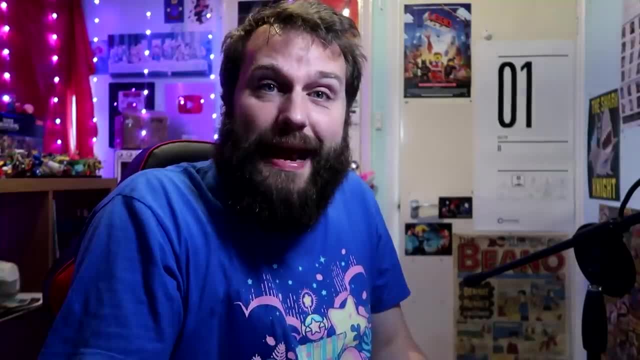 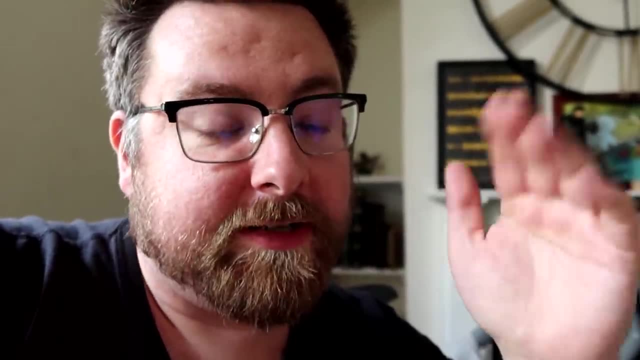 I can't do this. I can't do this. I'm a dog baby And I'm wet. Okay, I'm gonna make a board game. Alright, I'll admit, I am starting this episode with a little bit of an advantage. 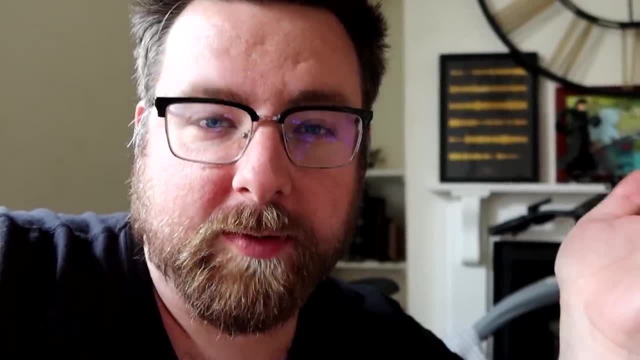 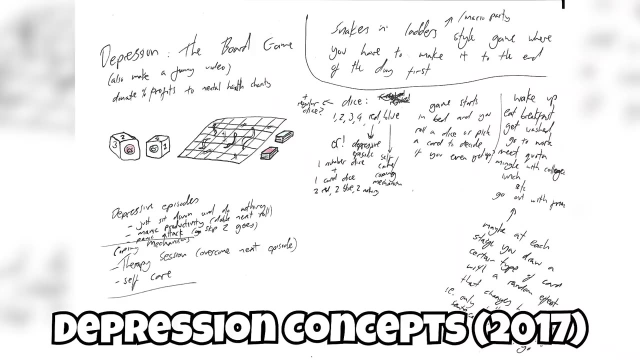 because I have depression. the game, Depression. the game Before we made Muffin Time. this is Muffin Time. it's a game that me, Eddie and Elliot made. I originally pitched a game, or was going to pitch a game, to Big Potato, the publishers. 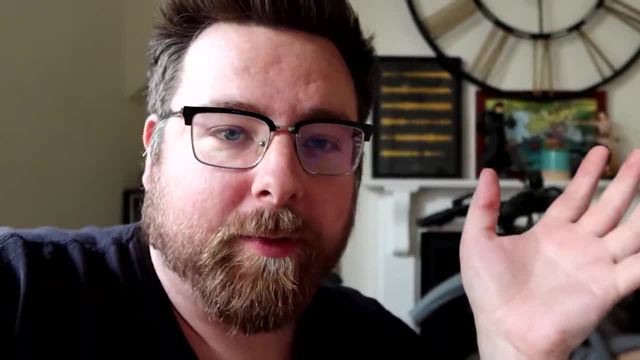 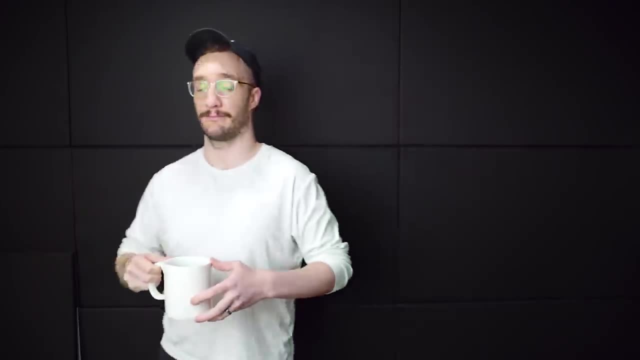 called Depression, the Board Game which was gonna be kind of like a dark comedy snakes and ladders-esque game about mental health. And that's what I'm gonna do. Let's get to it. I am gonna fix the Pokémon Trading Card Game. 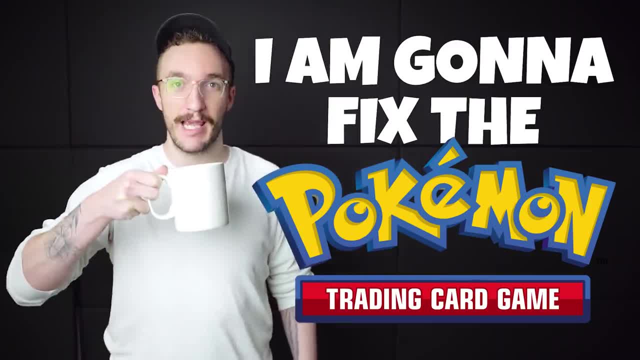 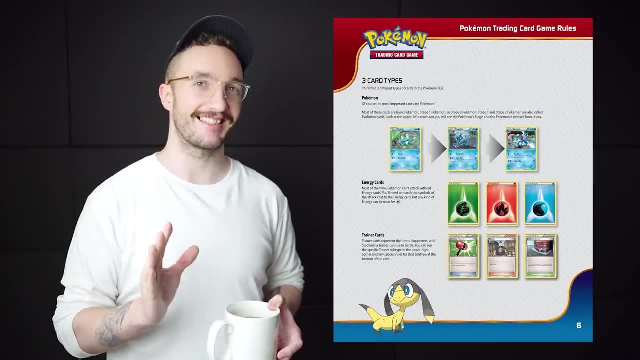 That's what he does, right? He does a little dance, Some text. You get the reference. yet I love the Pokémon Trading Card Game. I was such a huge fan of it as a kid, but I really didn't understand how you play it. 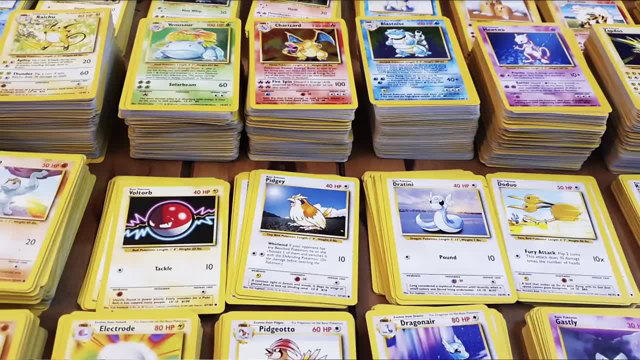 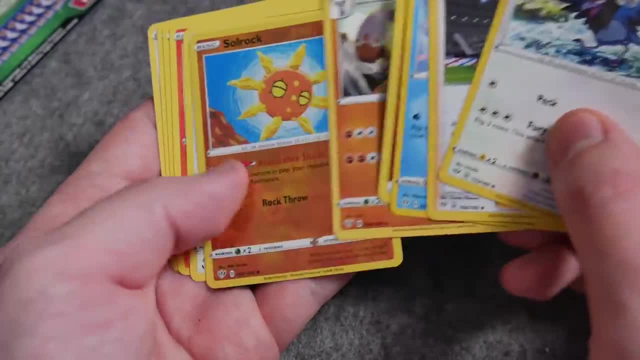 I loved collecting. it loved all the Pokémon cards. I liked having them in my little folder, But playing it was a whole other thing. All the health points, all the item cards, all the trainer cards, all the energy cards. There used to be so much going on, to be honest. 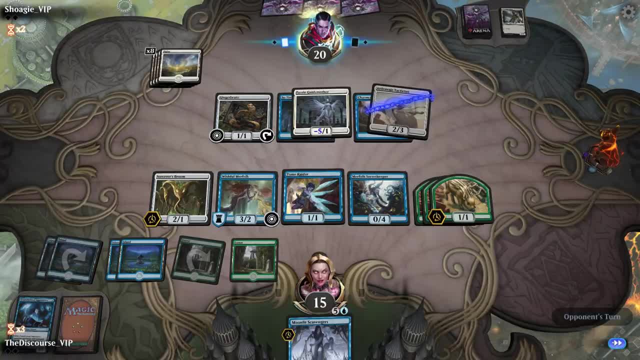 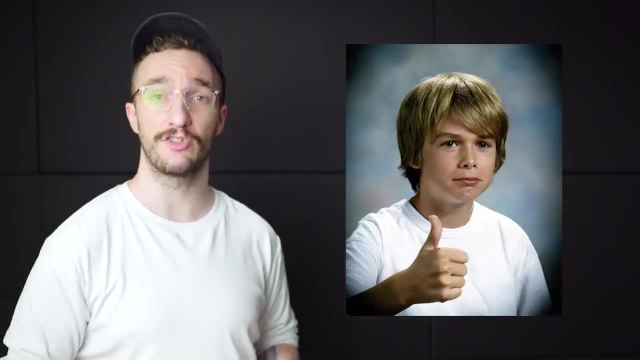 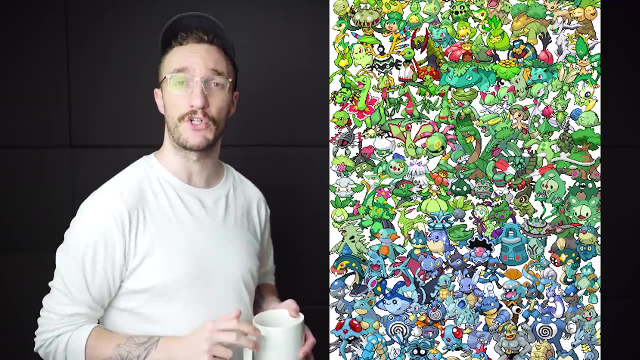 I know it's based on Magic, which is also a very complicated, hard-to-understand game. So what I'm gonna do is try simplifying it, Make it kid-friendly. You know the target audience for most Pokémon games, So it's an understatement to say that there are many Pokémon in the Pokémon universe. 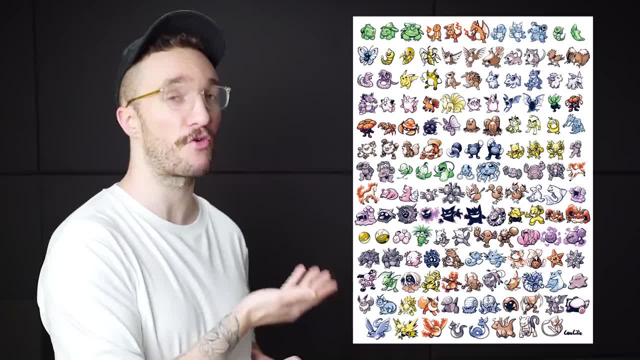 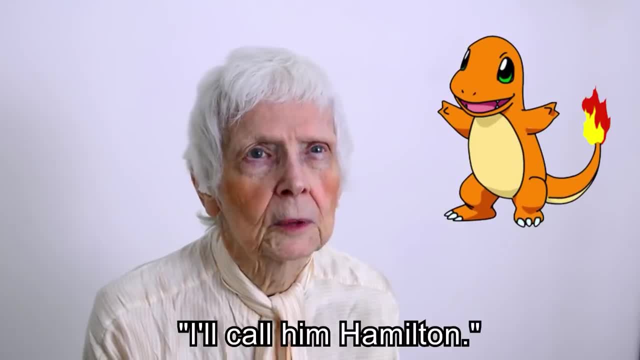 But for this- I'm gonna again simplify it- I'm gonna use the original 151.. I know it, you know it, everybody knows it. Even your grandma knows what a Pikachu is. I'll call him Hamilton, Easy right. 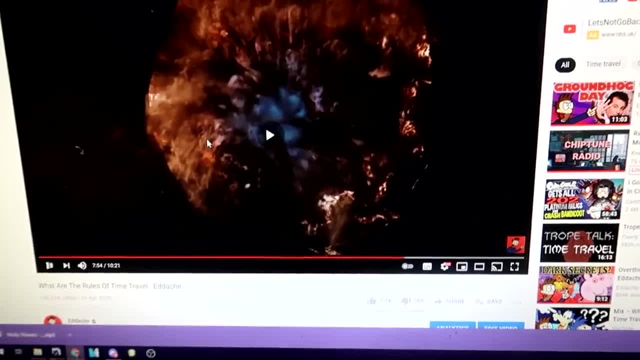 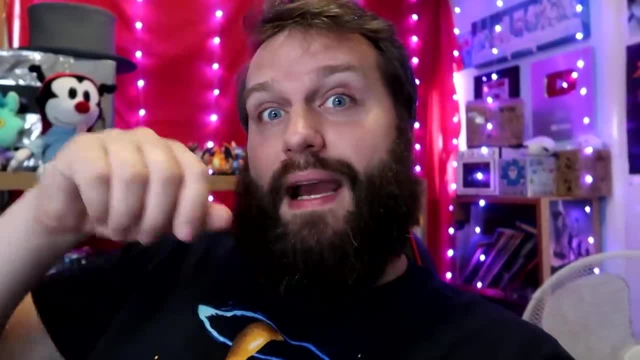 So a year ago I made a video about time travel. Part of it included this recurring joke about killing your granddad. I'm making a game about that, About going back in time to murder your granddad. I'm still working out the general premise. 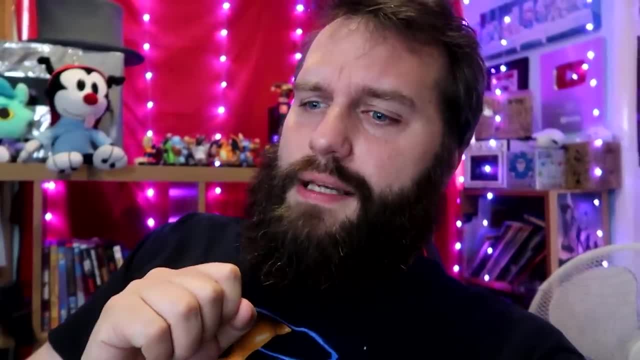 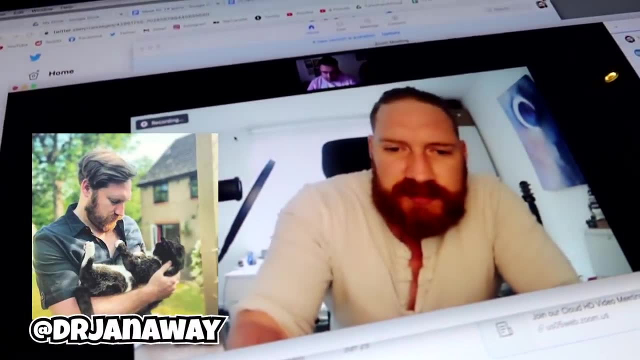 There's a bit of maths involved And I'm hoping that's not gonna be too complicated. But will it work? That's what I'm gonna try and figure out. So yesterday I gave a fella by the name of Dr Benjamin Jannaway a call. 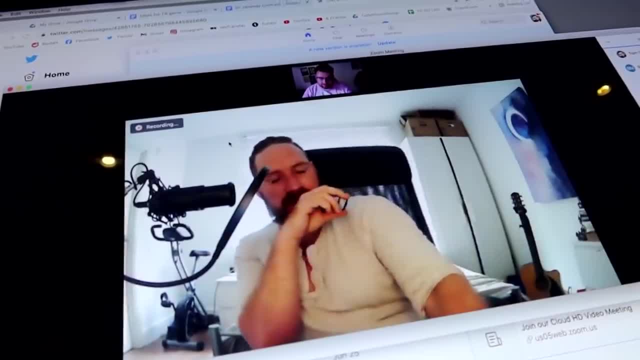 I had a little interview with him about five years ago about mental health And he said, hey, if you ever want to do anything else mental health related, give me a call, Let me know. And I said, okay, And then I didn't. 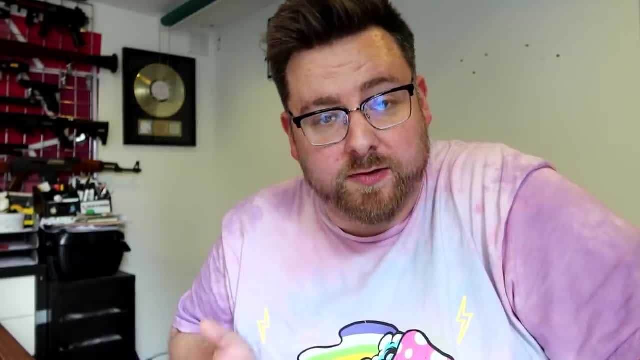 Because I had nothing to work on. But now that I'm doing this game, even if it's just for this stupid video, I want to do it right. You know, I could make a game about depression. that's, you know, sort of anecdotal and just like. 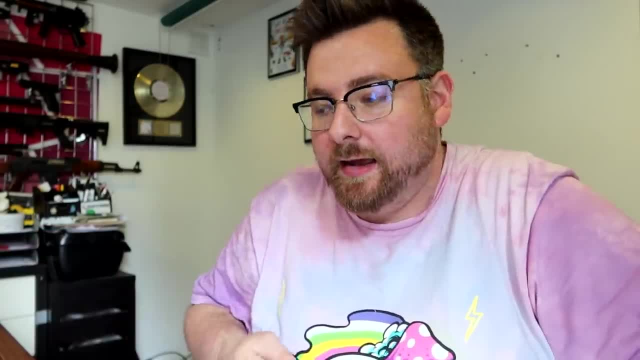 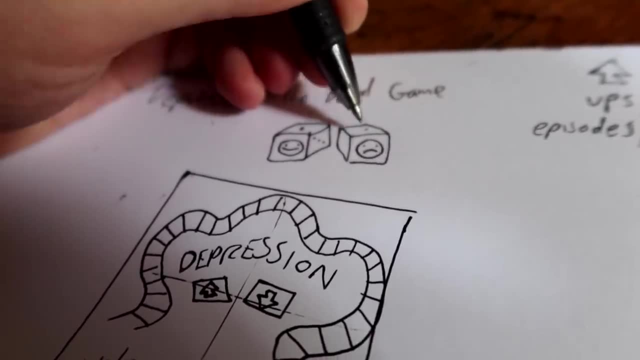 Oh, you didn't take a chance. You didn't shower today. Go back a space because you're stinky. Even if I'm just doing it for this video, I want to create something that is more helpful than harmful. It's inevitably going to be a bit edgy and offensive, because it's a ridiculous concept making a game about depression. 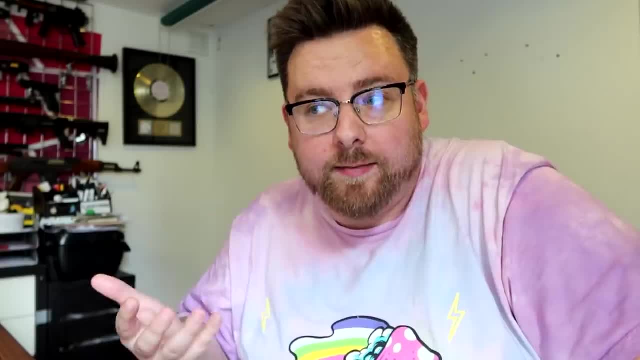 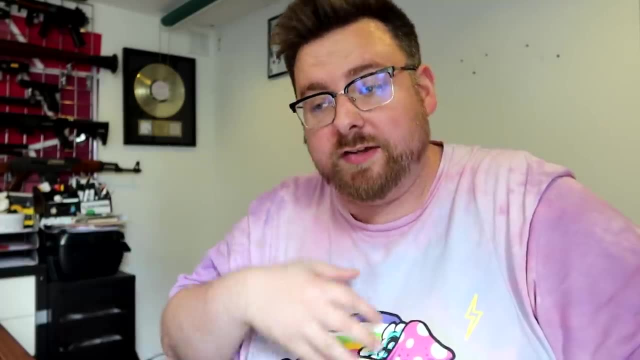 But I want it to be accurate and a game that someone could play with their family that would help that family empathize with what they're going through and what they need, Or, if nothing else, just normalize the experience. I don't know. But either way, I want to work with a professional who can help me get it right and also maybe reel me in. 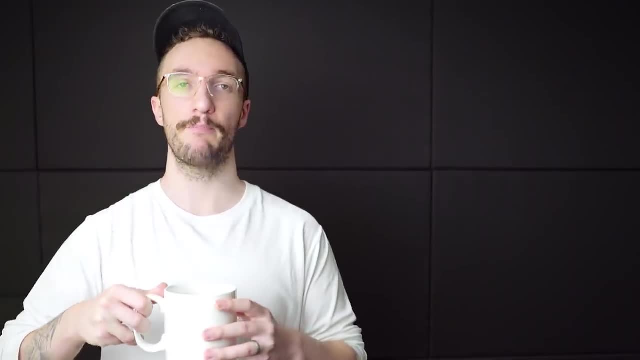 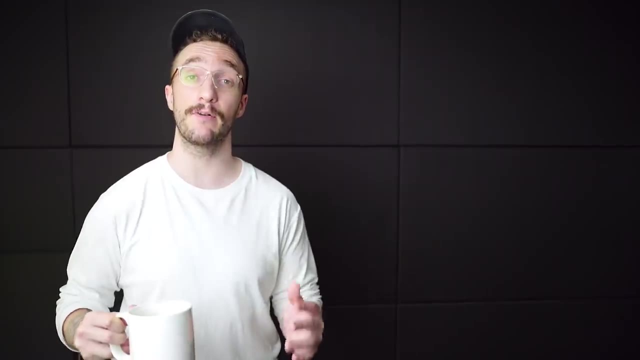 If I start to go A little bit too edgy. Oh now, a key part of any good game is balancing. Not like this, Not like doing this. No bad, stupid, I'm talking about game balancing. and boy the Nintendo fuck up the original 151. 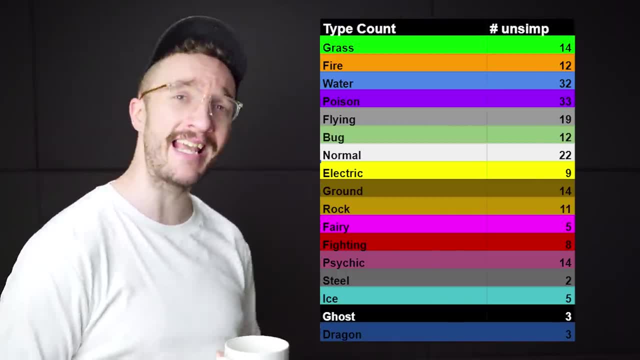 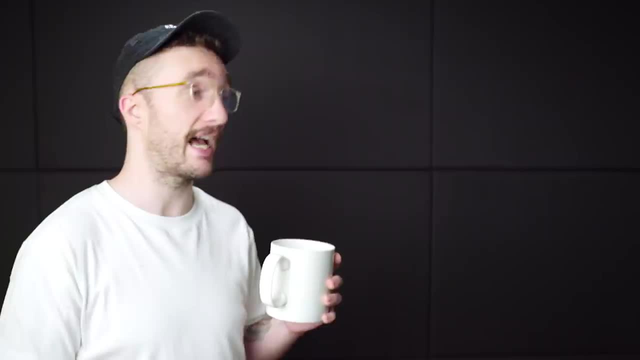 Look how many water and poison types there are. That's so many. What's going on, Nintendo? Were you reading too much Shakespeare? That guy loves poison. Loves to poison some people. I literally couldn't think of any other good reference for poisoning, but apparently Shakespeare loves to do it. 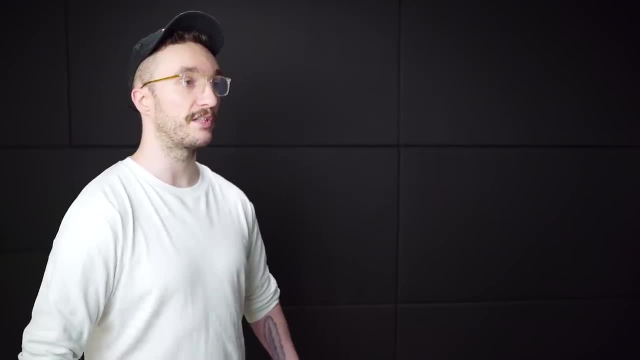 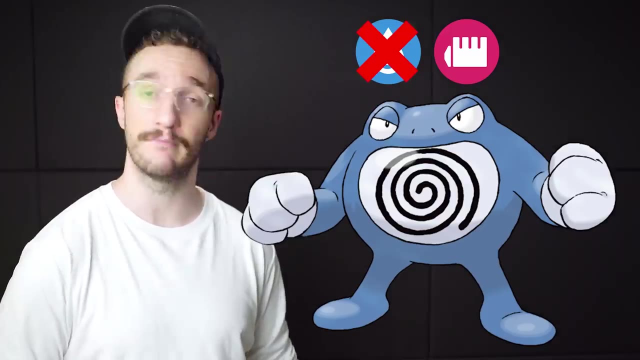 I've definitely read Shakespeare. Well, I guess it's up to me to fix this. Let's kill all the dual types, because I hate them. This thing really wants to fight me and I'm I'm scared. This is not ground, This is Rock Snake. 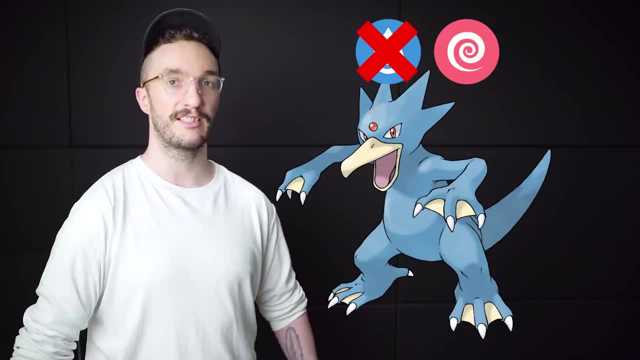 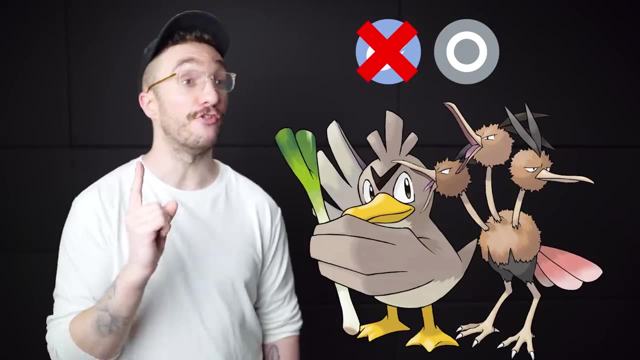 Ghosts can't poison people. Idiot Gold Duck and Psyduck are psychic. now It's in the name. Bats don't poison people. People poison people. I have never seen these fly. These are land birds. These are just eggs, but there isn't an egg type. 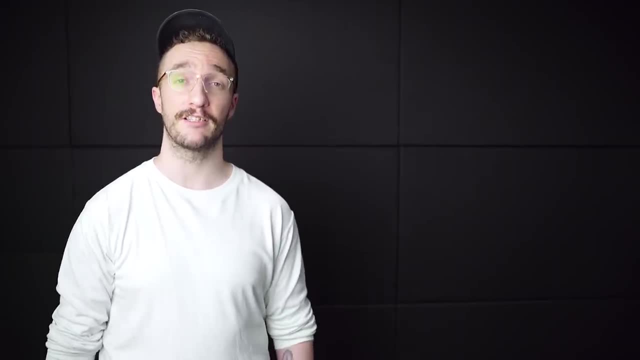 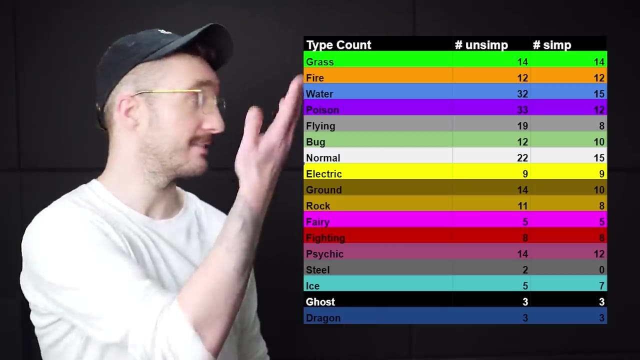 So it's grass, I guess. All right, Now that I fixed all of Nintendo's mistakes, Let's see what the chart looks like now. Wow, So much better. This is literally the best I could get it, and it's a lot more even now, I guess. 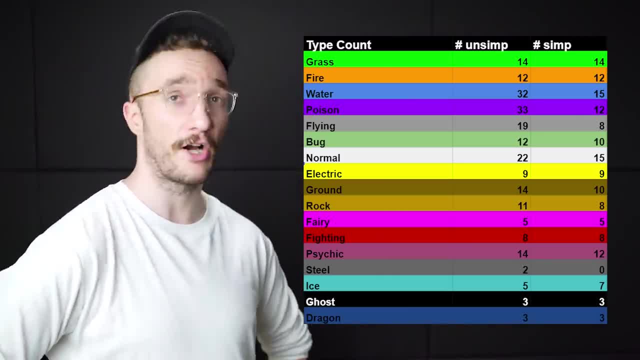 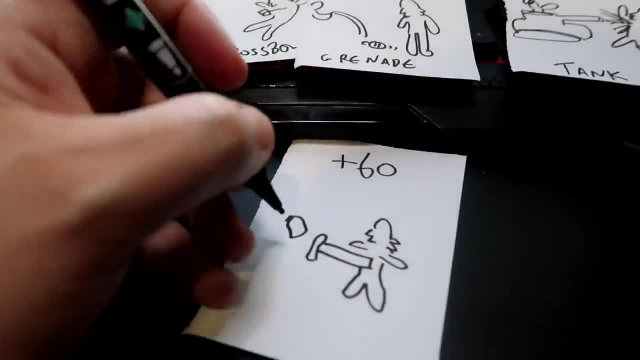 But I have to say goodbye to steel. Sorry, steel, You got to go Boosh, You're gone, All right. So I've created a bunch of cards, different weapons and even some duds, So maybe we should give this a test. 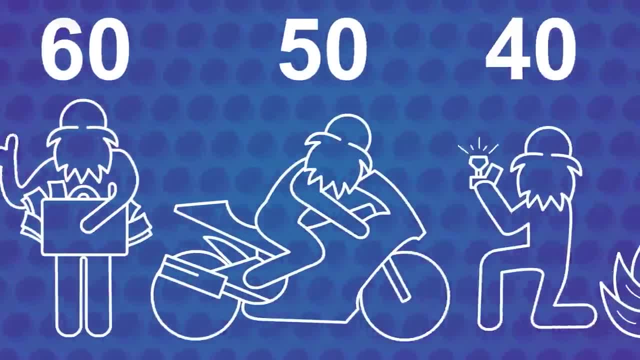 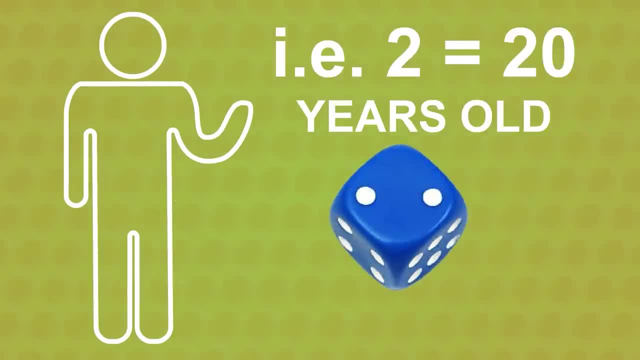 Granddad is 100 years old, So you need to jump back through the decades, killing him in any error. But the game is not one until baby Granddad is dead. before the game begins, Each player needs to work out their age. If you're in a decade where Granddad is still alive, you can try to kill him. 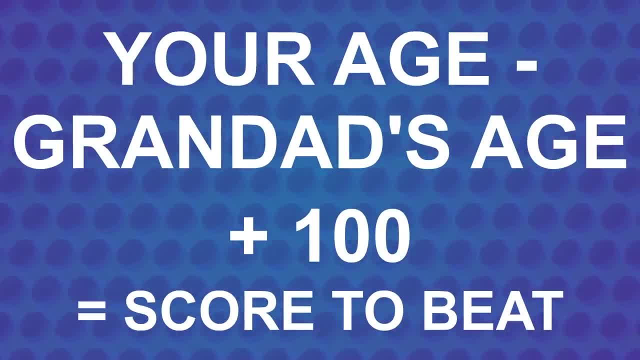 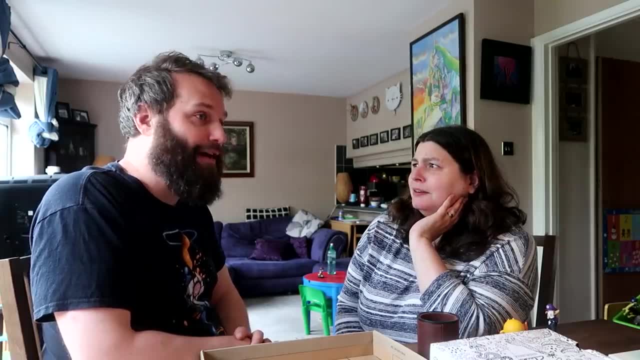 Any attempt on Granddad's life must be calculated as follows: Your age minus Granddad's age plus 100.. So let's kill Granddad. Why do I have to kill a baby? Because it's your granddad. Can't I just kill him in the war, or something? 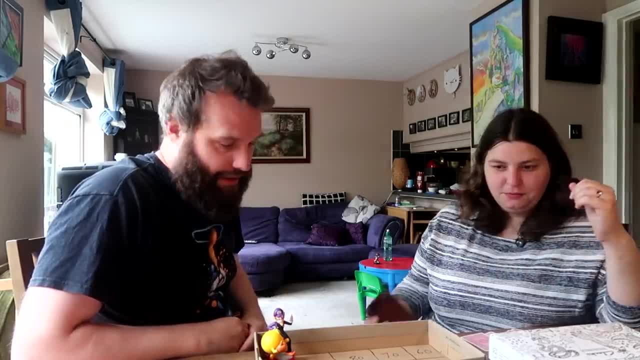 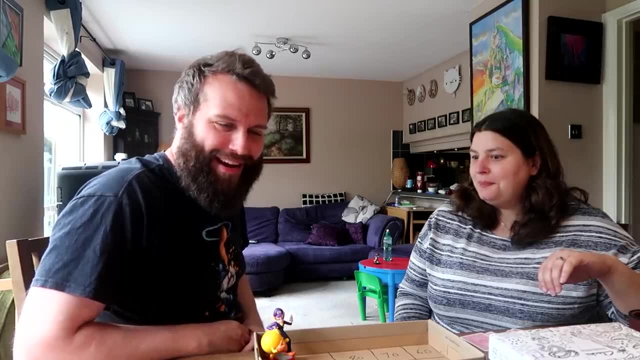 That would have been easier. I guess you go first. Okay, I want a weapon. You're going to just go right ahead and take a weapon? Yes, I don't think there's much point to me doing anything without a weapon. I kind of don't want you to take a weapon right now. 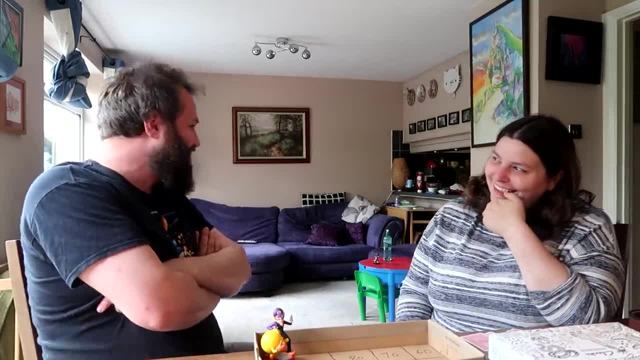 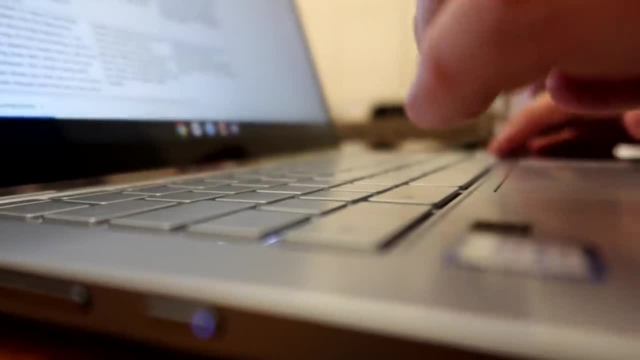 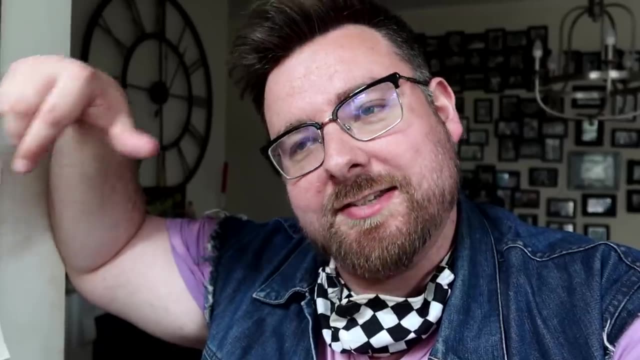 Shit, Is that an immediate game breaker? Yay, You killed baby Granddad. I put together a little list of depression symptoms that I wanted to include into the game- I guess anecdotal and stuff- and Dr Jannaway kind of just kind of just pointed out a few of them and said: those, those aren't really depression. 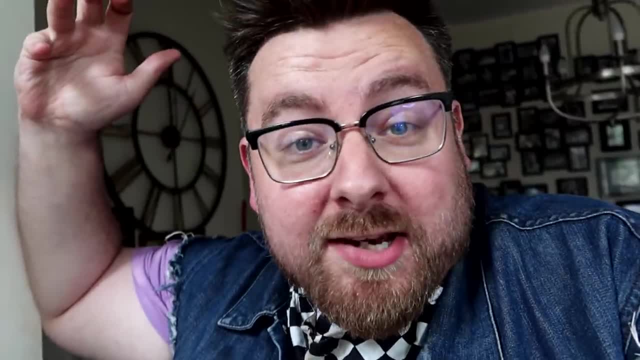 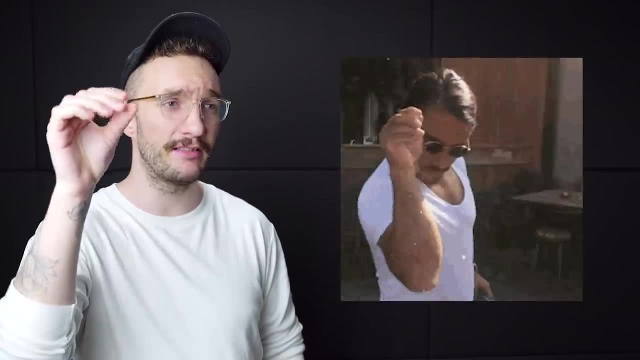 Those are ADHD. So I have two excuses not to get anything done now. All right, Now that the foundation is sorted, It's time to add a bit of fun and games. Add a bit of spice to the mix, Add a bit of muffin time to it. 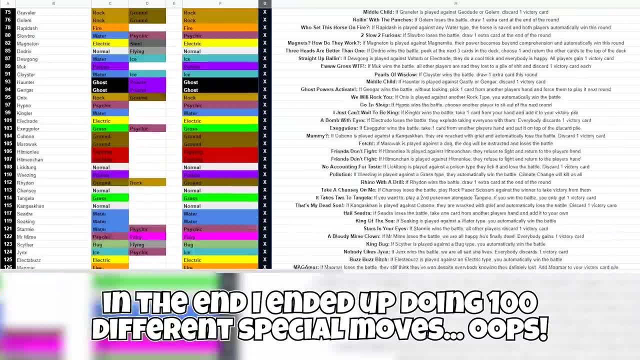 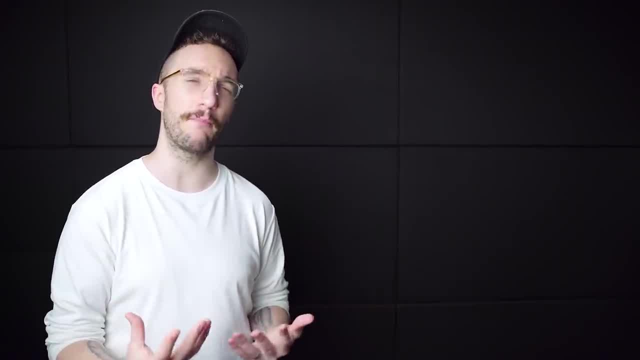 You know, and a bit of chaos, chaos. So there's 83 different funny moves in there. now Will they all stay to the end? I don't know. part of me thinks that might be a bit too much, And unfortunately I'll never be able to know if I've done too much or too little. because the first 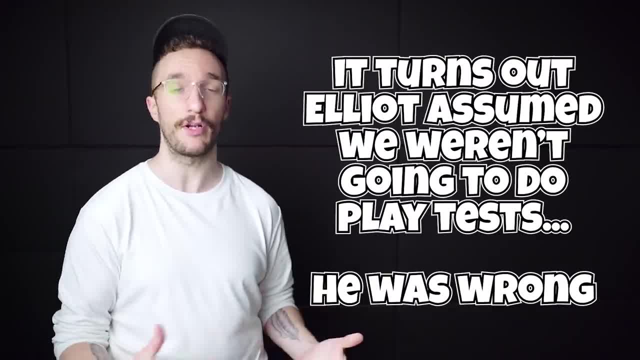 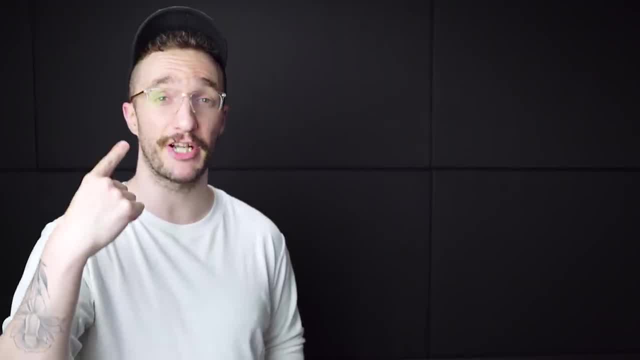 And only playtest of this game will be with Tom and Eddie when we wrap up this try hard episode. So, yay, I love pressure. That's probably what this is. It's a bloody pressure headache from all the stress. So let me tell you some of my favorite moves, some of my favorite special moves. 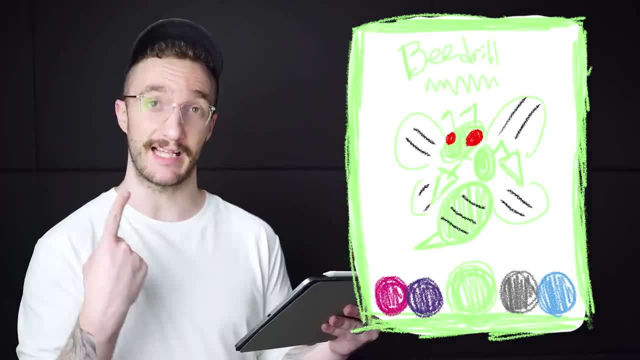 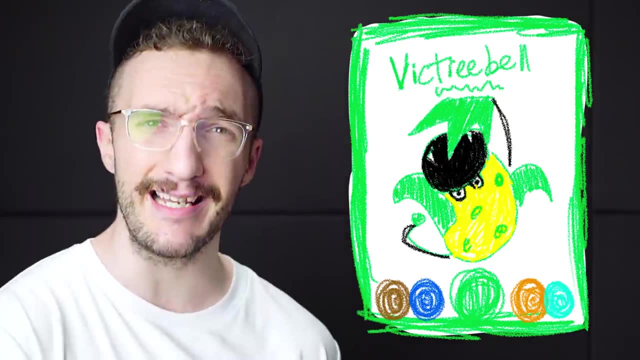 There's a bee, and that is if be drill is played against Elliot- That's me- He automatically loses the round, because I'm scared of bees more like Victory Bell. You get it. if Victory Bell wins the round, draw one card And add it to your victory pile. 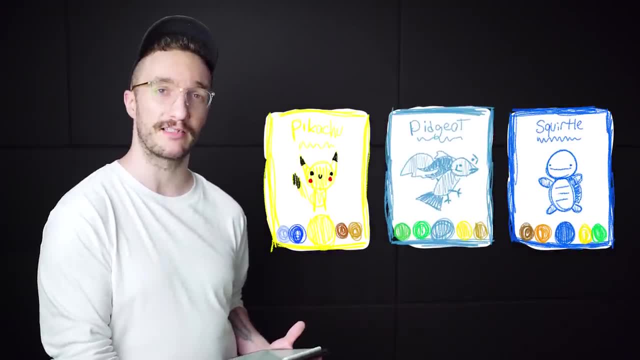 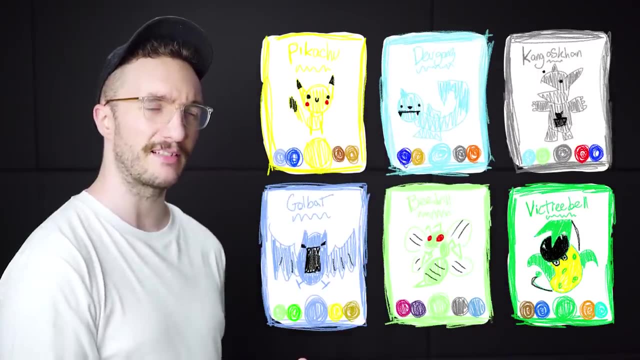 That's something I don't think I've explained yet. in my mind You all play one card at the same time. You decide who wins and whoever wins adds that card to their victory pile. in my mind It was like six maybe, because that matches the amount of Pokemon you can have in your party in the Pokemon games. 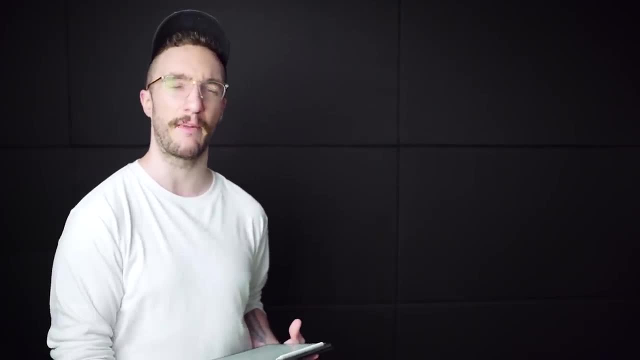 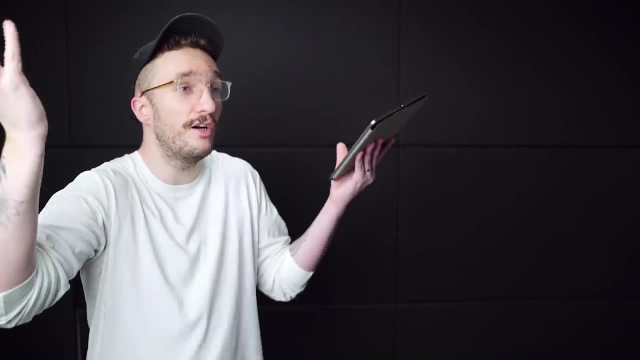 I'm worried that I'll end up making the game way too fast. So I might increase it to 10, which is, I know, very muffin time with me, but it's a good around number in it. but it's going to be hard to work out because there's no beta testing or anything. 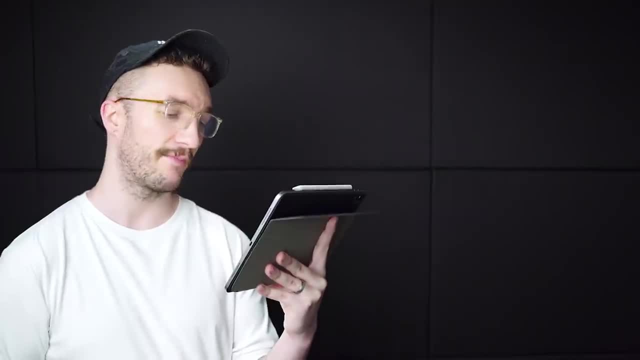 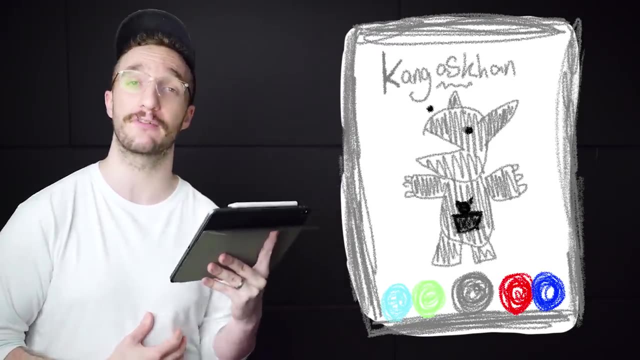 So I'm just going to have to guess. and last but not least, One of my favorite cards is that's my dead son. If Kangaskhan is played against Cubone, they are wrapped with grief and automatically lose this round. sadness and despair. 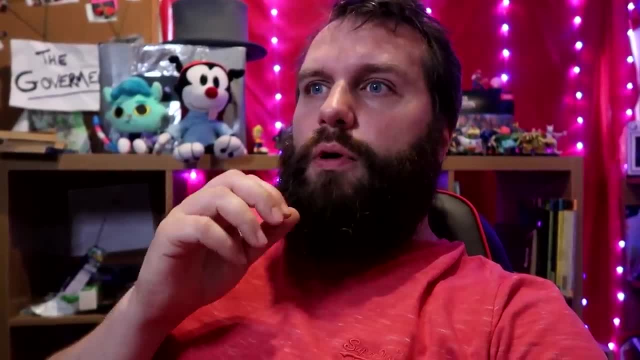 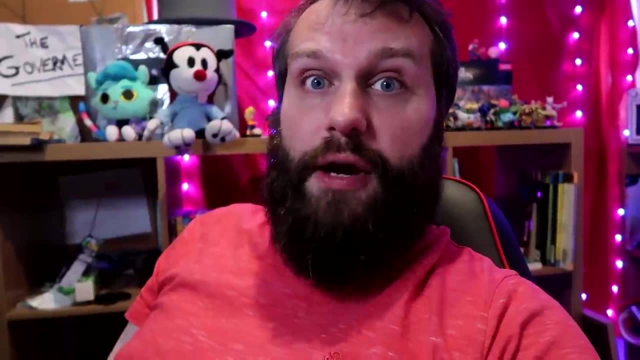 It's within us all. I'm going to spend today working more on the design of the cards. I've come up with a list of brand new weapons, stronger weapons. I've got some cards I'm going to draw the weapon designs on to. I've also got some tokens and dice. 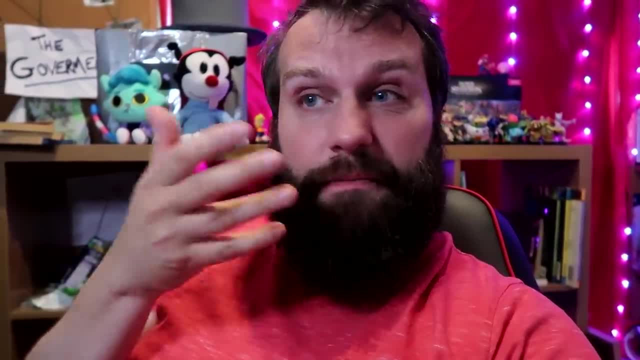 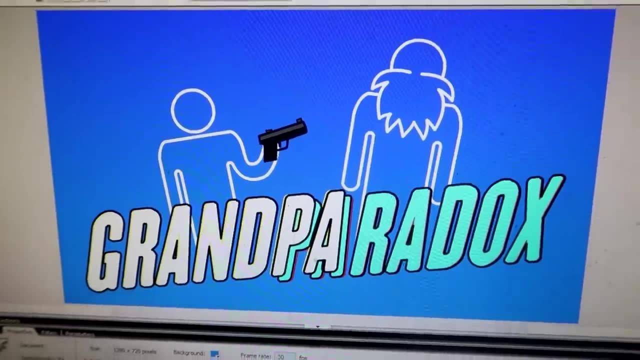 So I'm getting stocked up. So now I guess I'm just rolling into making it pleasing to look at Game. Oh, and the best part, I've got a name for it Now. it is called Grand Paradox. It's like grandpa, but Paradox. you see it's, it's a mix of the words. you see it's, it's work. play. 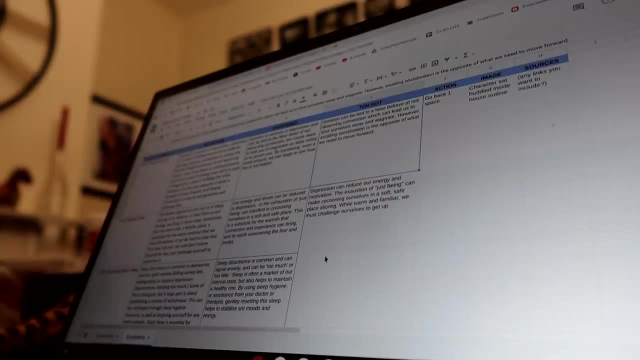 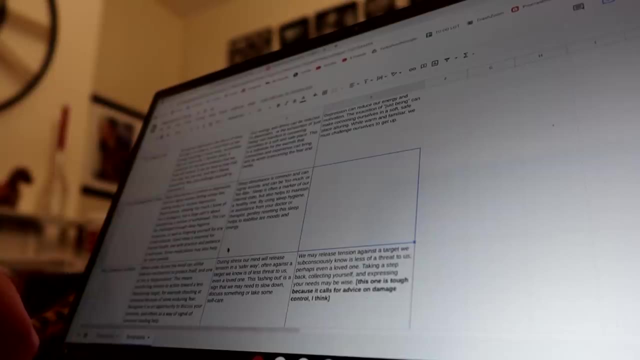 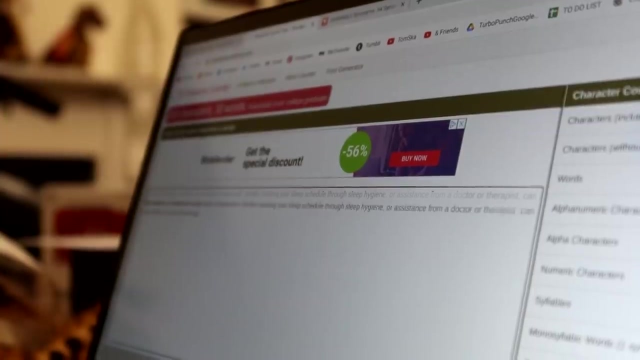 So it has been a very busy few days. I worked with the good doctor Jannaway to put together a list of like 70 depression things- you know, bad things the depression does and good things that can alleviate depression- and packed it full of information that will hopefully be helpful to no one. 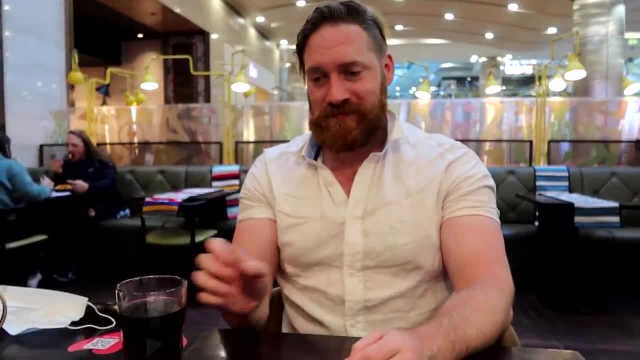 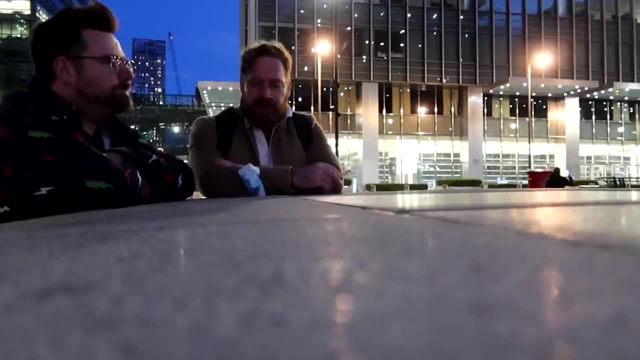 And then I met up with him and we talked about really fun stuff like self-harm and suicide, and if we could even broach that in a game like this, could we give it the reverence it requires, and we kind of settled on: no, No, you kind of can't, so best not to, even if it is a potentially significant factor in depression. 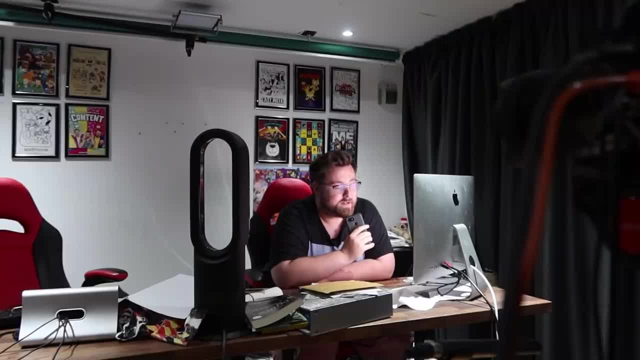 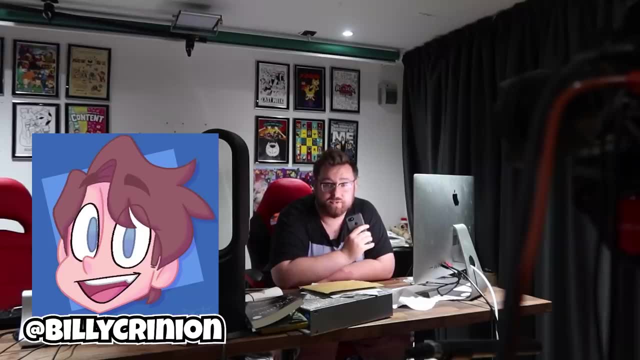 Don't run the risk of causing more harm than good. And then, finally, I started working with Billy crinion on illustrating the cards and he put it all together and I noticed it was a lot of dudes, just a lot of dudes. when you're drawing in an ass of style, 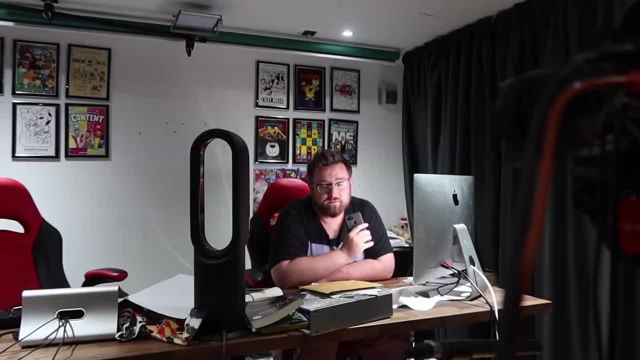 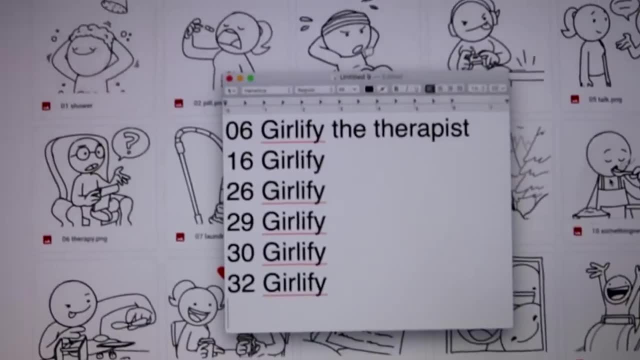 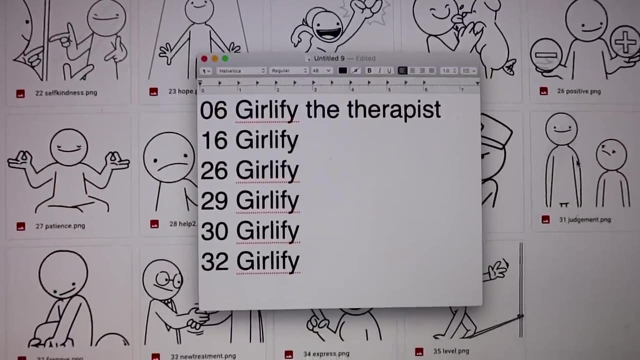 or I think when you're drawing anything, it's very easy just to draw yourself, to draw guys, unless the character specifically calls for it Otherwise. so we went through and girlified was my a very technical term- A lot of the cards to make the game actually represent a diversity of people. 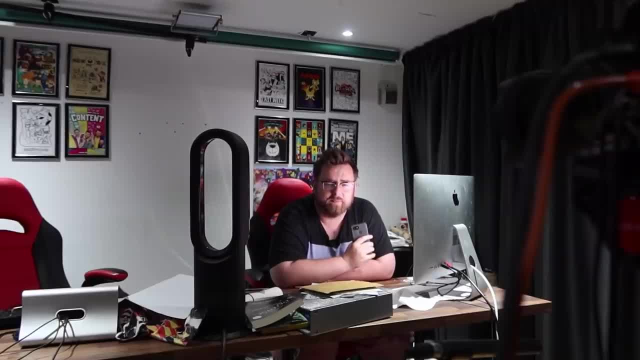 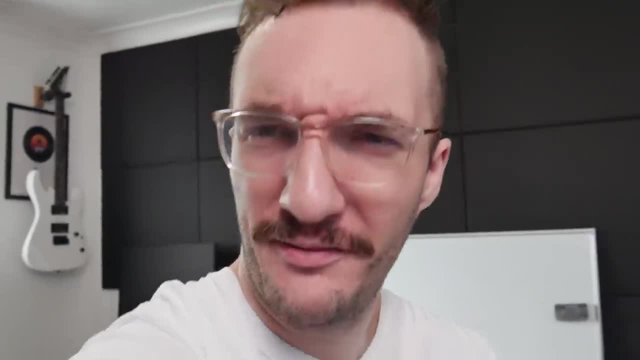 because I want that to be important for the Eddie and Elliot who are playing this game. It is 1 am. What am I doing? This is my rough idea of what I'm going to try go for so my initial idea for the art of these cards. 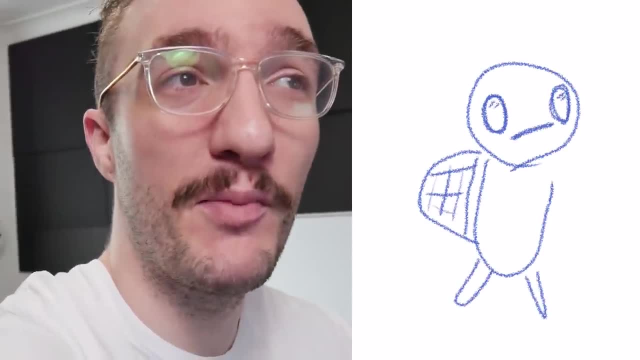 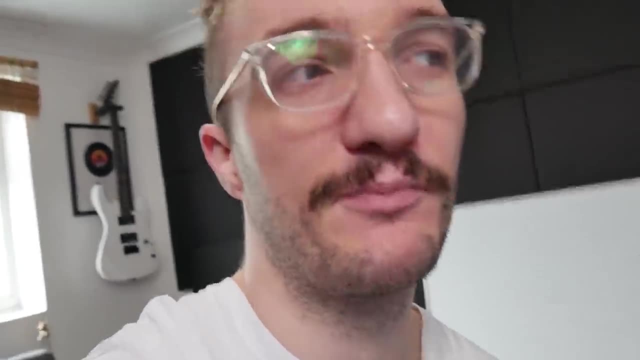 was to make some funny content by redrawing all the Pokemon cards at my best ability. I'm not a good drawer, So it'll be very funny, I think, but because of how strict the deadline is on this, I'm going to just initially steal a bunch of things from online. 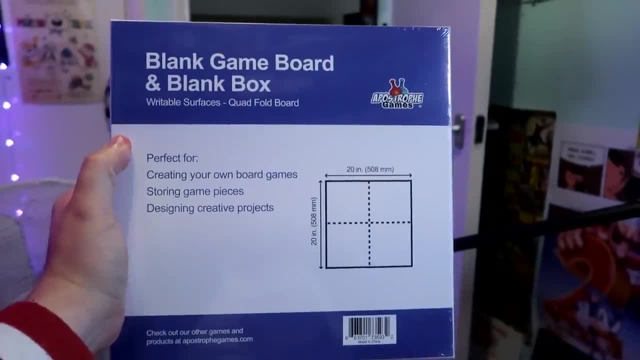 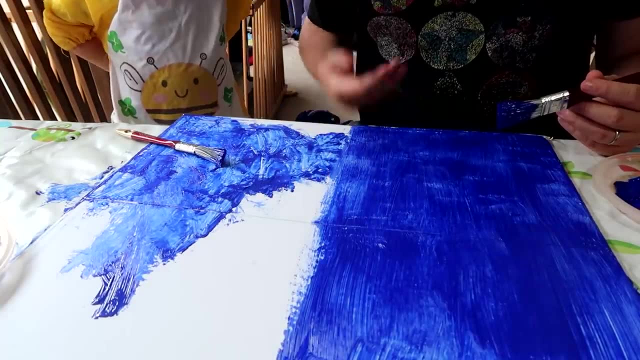 Yeah, my favorite board game: blank game board and blank box. Hello, We're going to do some painting. Are you sure you're finished? Well, I mean, yeah, I mean you just compare the two, you can clearly see that you're clearly finished. 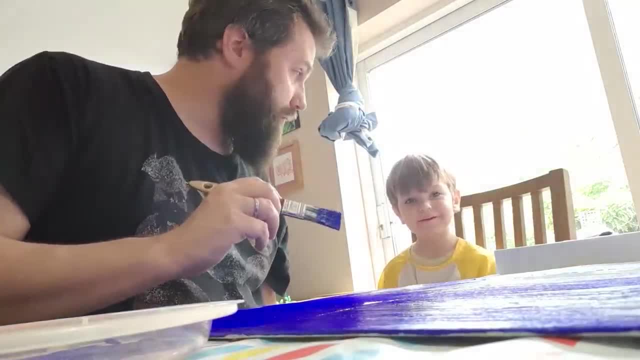 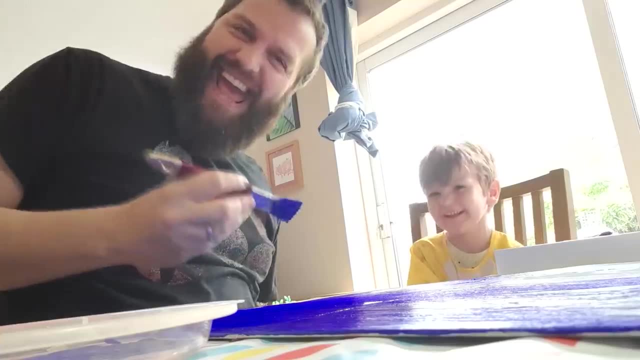 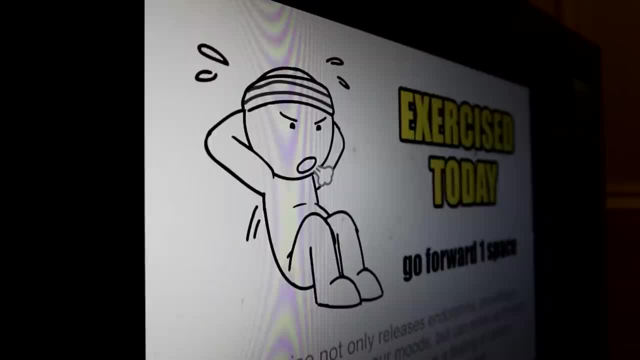 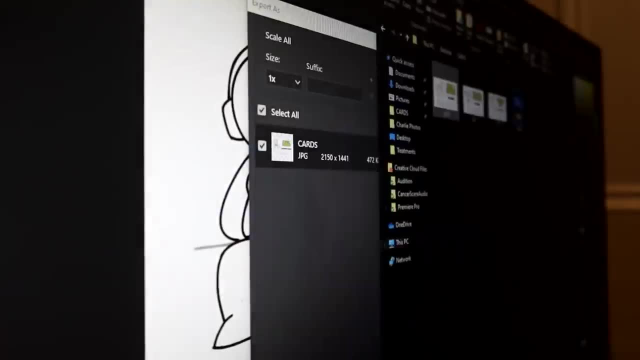 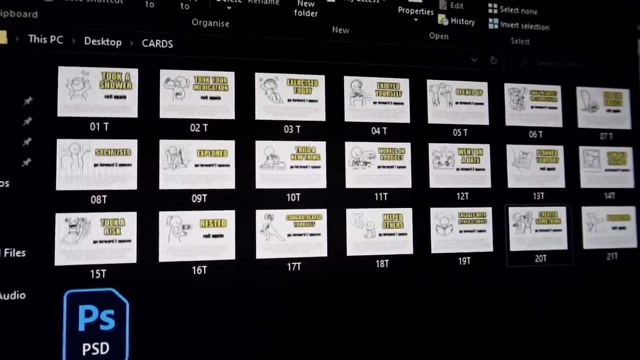 Oh my God, You know what I do not envy Elliot having to do this some 250 times over and over again For muffin time. This is a fucking nightmare. I'm tired and I'm very bad at this. I've done about 21 and I've been working at this for hours. 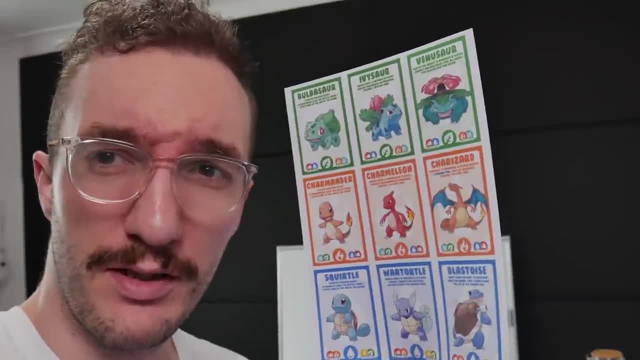 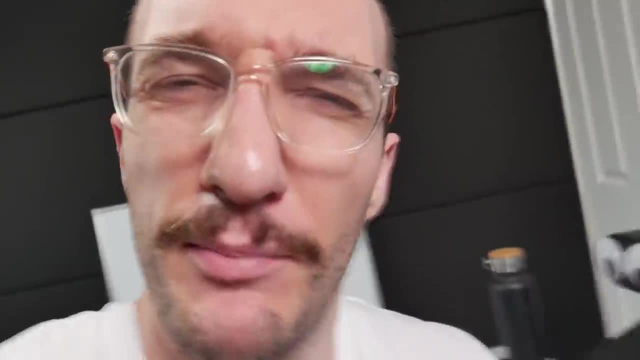 So here's the first test. print is very muffin timey. I understand that I'm going for that kind of vibe, though I think they look really nice, I wish I could get them, like, properly printed so they could actually look as good as they are right now. 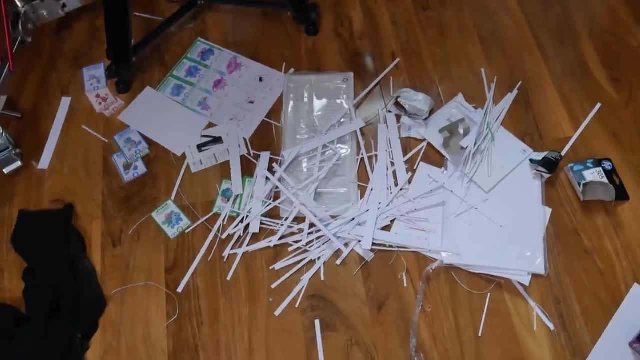 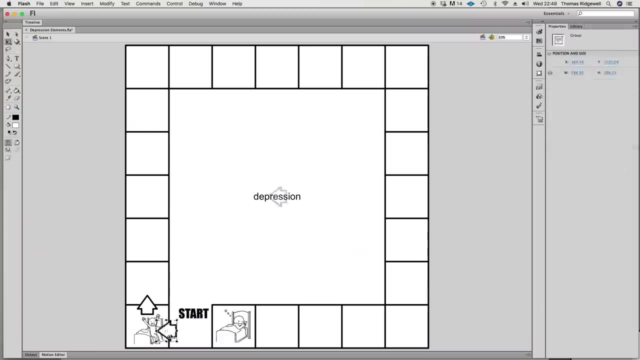 But sadly this little printer is just going to have to do. Look at the mess I've made. So here they kind of are. Overall I think they look pretty nice. Just spent a few hours putting together board design options. Pretty hard not to just reinvent Monopoly or Snakes and Ladders. 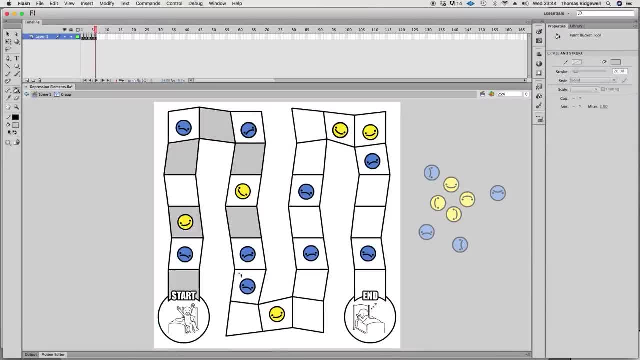 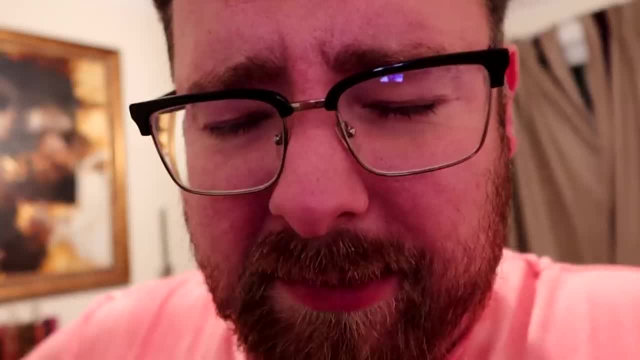 But that is done. now. I've exported all of the cards, I've formatted things, I've sent them off to the printers. I think I've done everything I have to do. I forgot the dice and the player pieces. No, What do you mean? you can't just buy one blank dice. 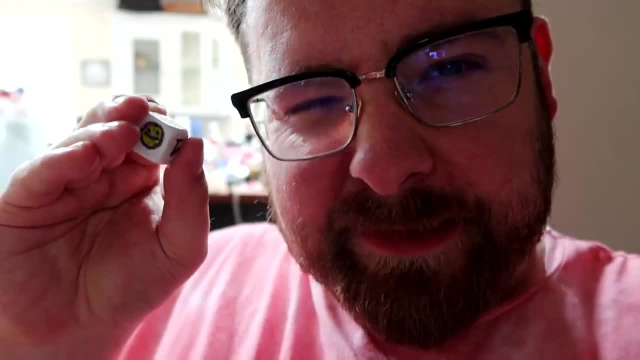 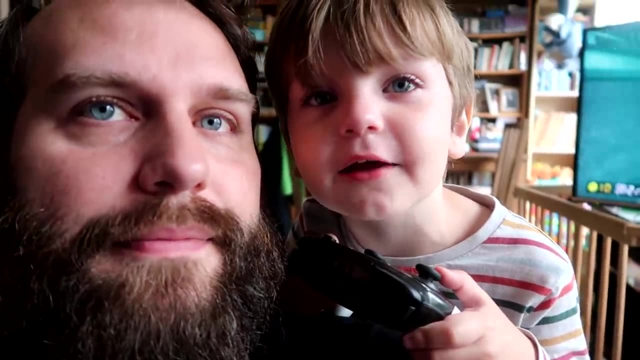 That'll do. It's the squad everybody. Yeah, I think I'm going to need some help on this dice, Meg. Yeah, Do you like Grand Paradox? I like Grand Paradox. There you go, Put that on the box. 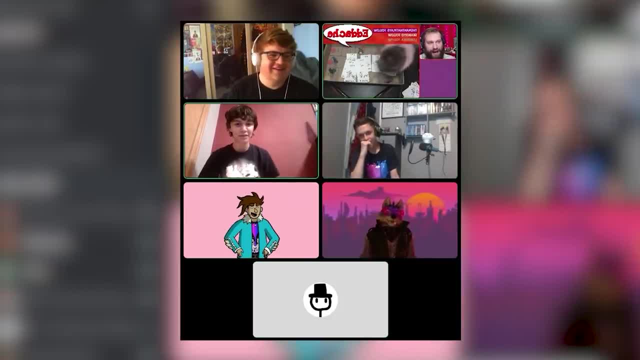 So I did some more play tests, this time with members of my Discord server, And it's a lot of fun. It's a six. Yeah, Grandad's dead, We killed him. Baby, Grandad's dead, Let's go, Let's go. 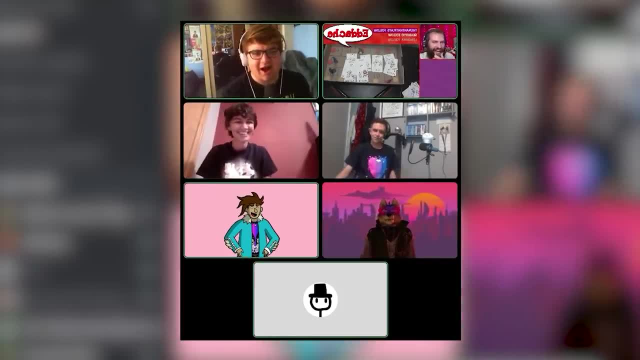 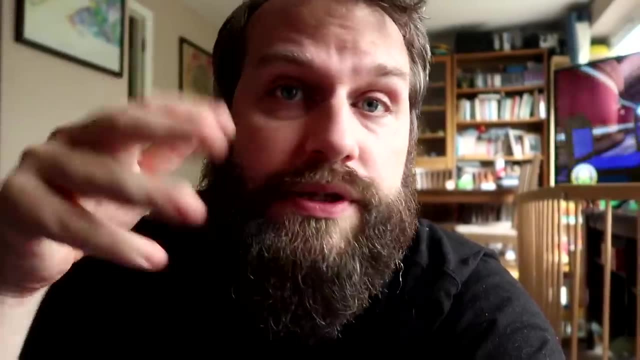 We killed Baby Grandad For FighterJet. Yeah, Good job, lads, Let's go home. It works with four players and five players, So that's brilliant news. It doesn't become too bloated with too many people playing. 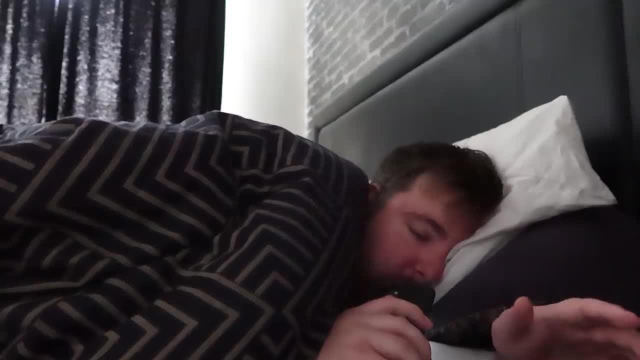 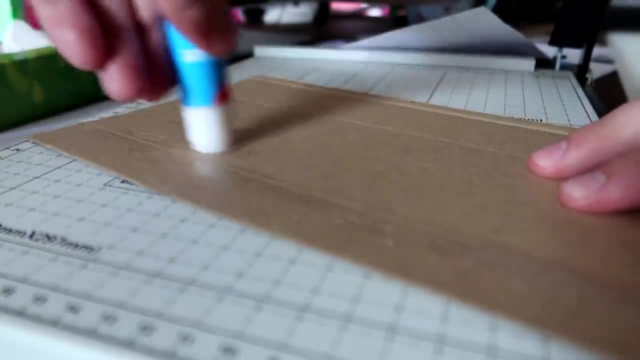 But the issue of balance is still there. So I got a lot of stuff done, Printed off a paper version of the game. Definitely didn't run out of ink a lot of times doing it, But stuck it to some cardboard and had an actual play test. 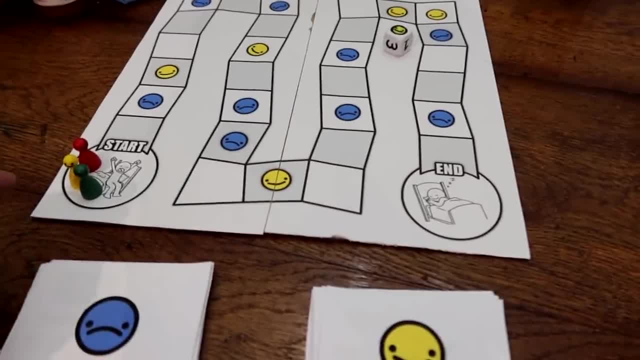 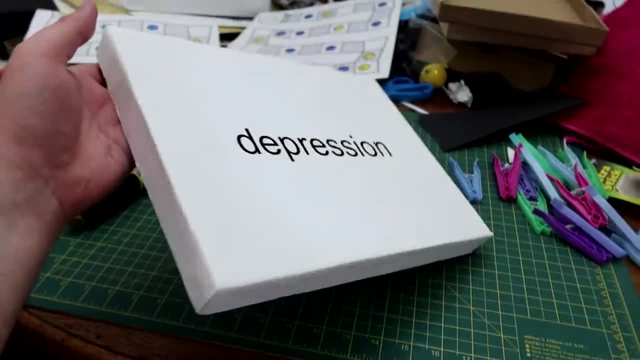 And the game works, which is really cool. I'm really glad. I feel like I could make it a bit more interesting, though, So I might redesign the board, Made a box, You know, cut it in half and glued it back together. 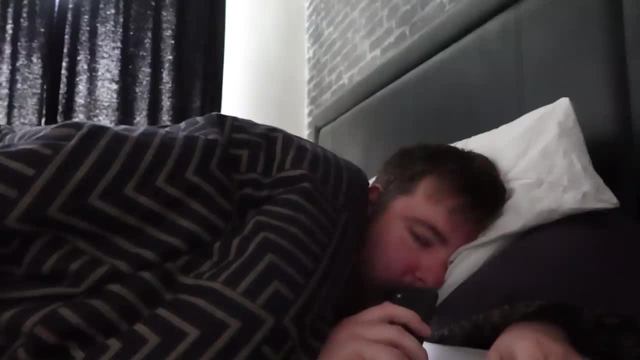 And it's a bit ugly, but it's mine. I'm really happy with it. But I will say maybe working on a game about mental illness, forcing me to think about mental illness a lot while circling the drain of a depressive episode, wasn't my best play ever. 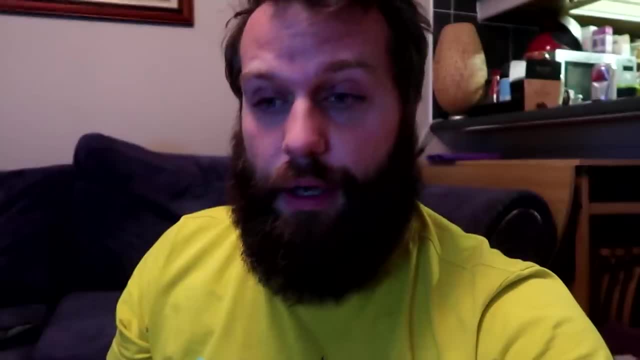 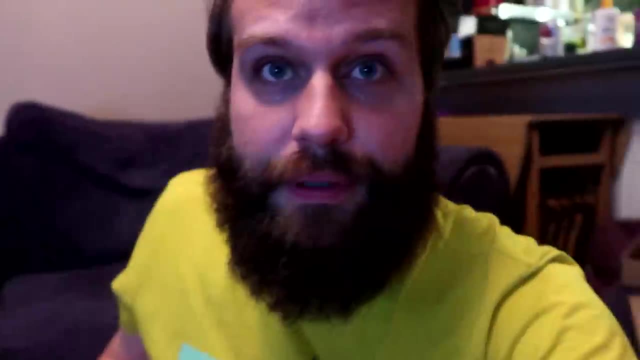 I'm not actually doing that bad. I just want to beat Bo Burnham. Okay, so I had a real bloody time getting these done, But they're done. There we go. Got some handsome stickers here. I'm going to be putting them onto the board. 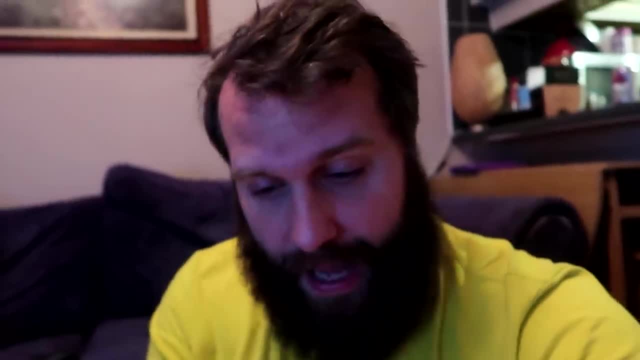 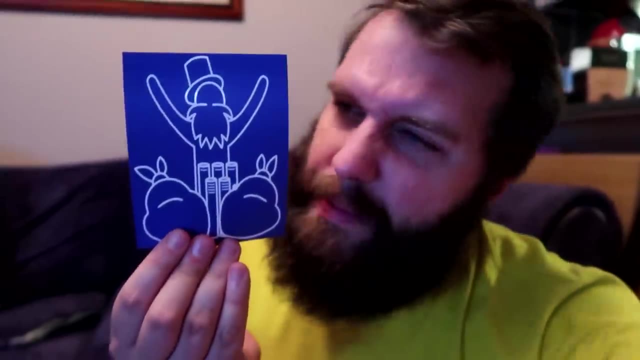 And it's going to be great. But let me show you exactly the problem I had. So here's an example of one. This here is Capitalist Grandad, A tycoon, as you can see, A little bit stretched, A little bit taller than I wanted it to be. 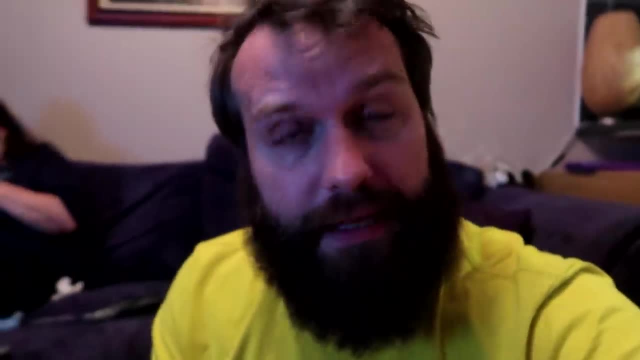 But you know it's there. There's the job. Now you might think that looked alright. How did they get that wrong? Let me show you. Let me show you. This is how they did it wrong. He's a bit wide. 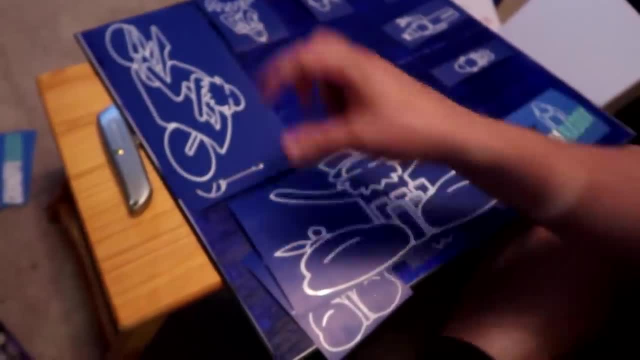 I mean, maybe it's not so bad. You know what, if I put that one there, Put the motorbike one there, Put that one there, That one there, You know, the child one there, You know it'll be a shorter game. 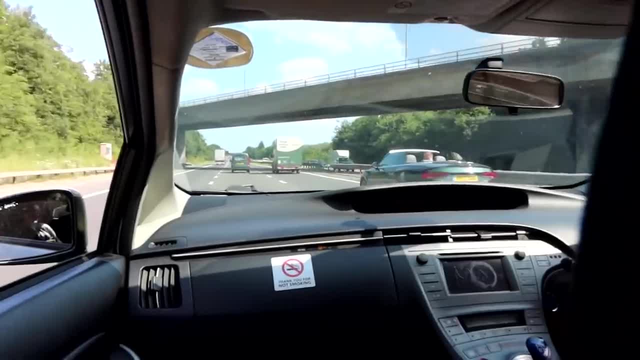 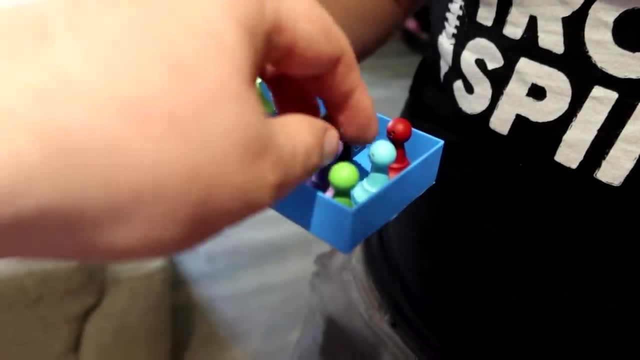 So I tweeted out asking if any of you had any experience making dice or figurines. And lo and behold, a fellow by the name of Ben aka The Iron Spine replied And he's just spent the past few days working on some figurines and a dice. 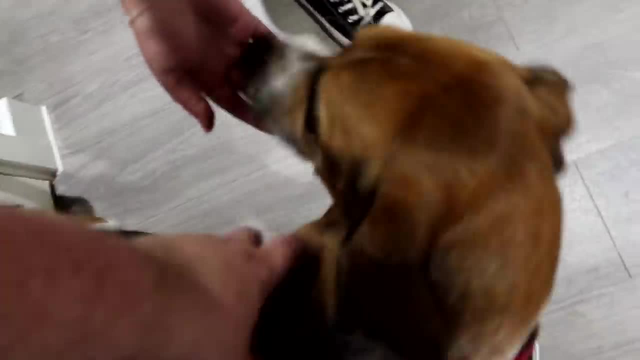 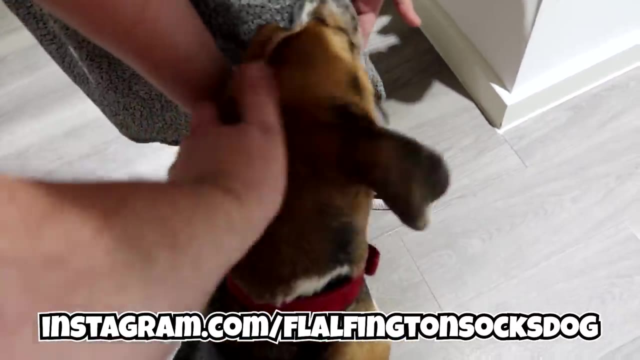 And I'm on my way to see how we did. That's so cool. He's internet famous already. Oh, really, On Instagram. Oh, he has an Instagram. Of course. Damn Ben's put so much work into making these pieces. 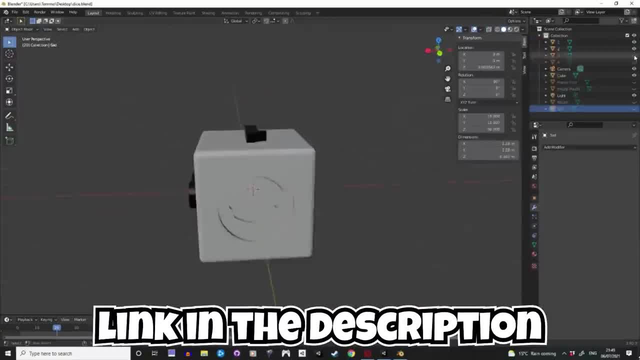 It's been kind of a nightmare And I can't believe it. I can't put it all in this video. I can't really put any of it in this video. So he's got a whole video on his channel, all about this. 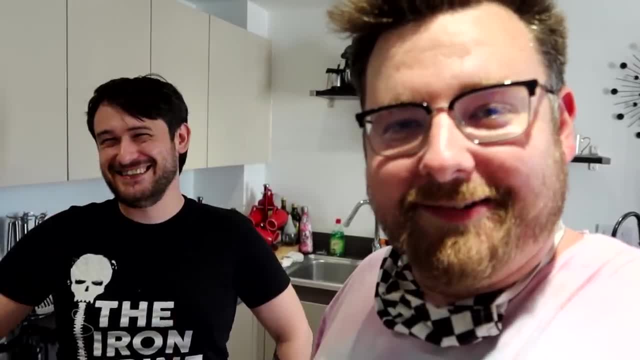 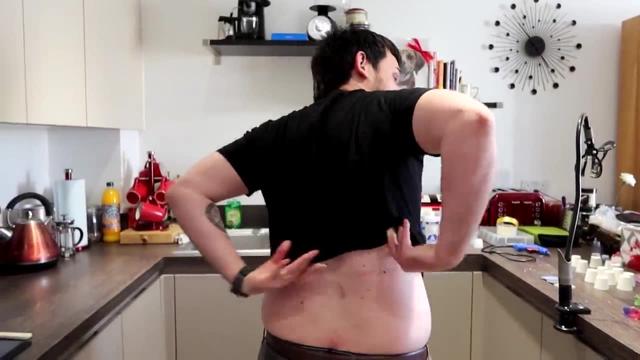 Link in the there. Thanks, Watch that. I'm so sorry. What do you mean? you have a battery. So I am actually a crippled cyborg and there is actually a battery in me. Whoa, Oh, that's. You can touch it if you want. 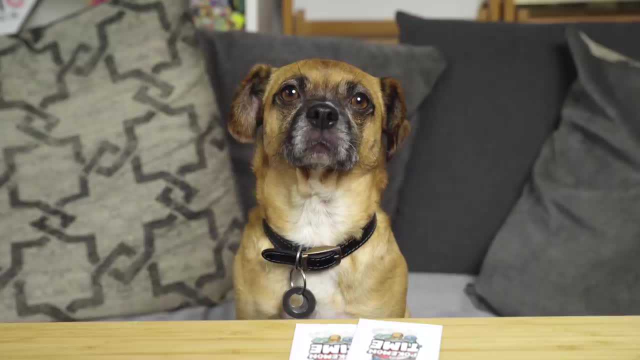 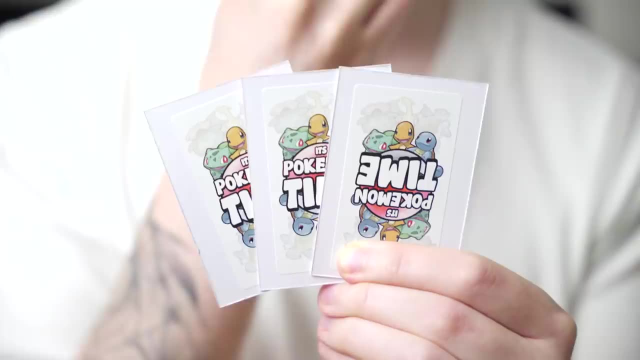 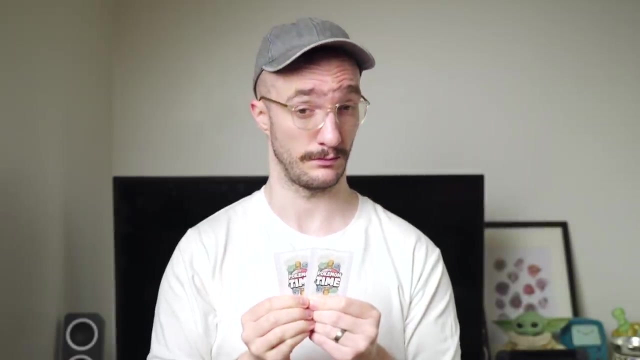 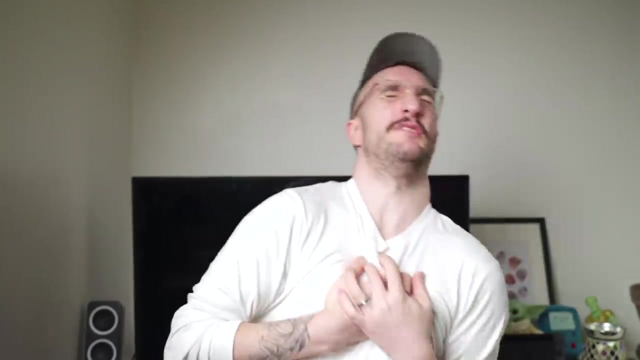 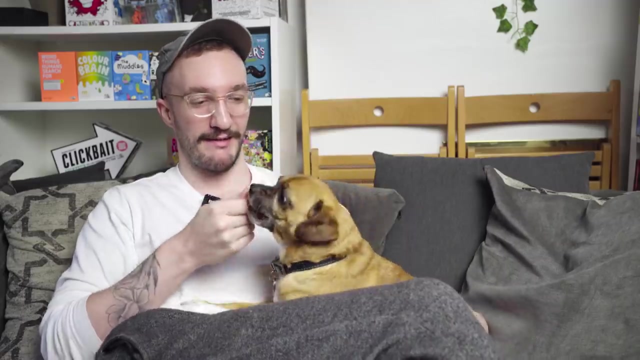 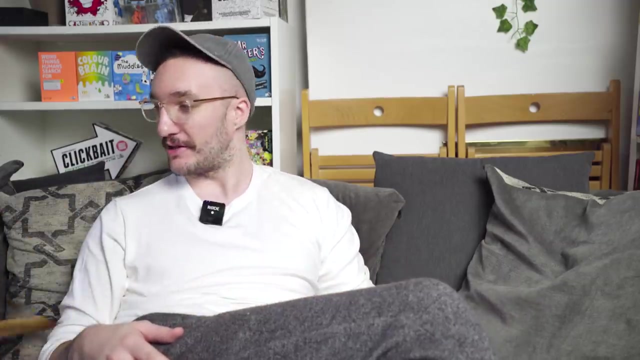 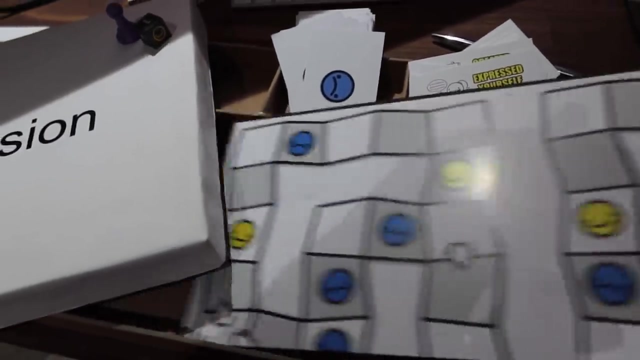 I'm good. I'm good, Cheers, Cheers. I'm so honoured you brought your battery and voted me out. Cheers, Cheers. Ready for some dog ASMR Gross. The game is done. I'm really happy with it. It's come together really, really well. 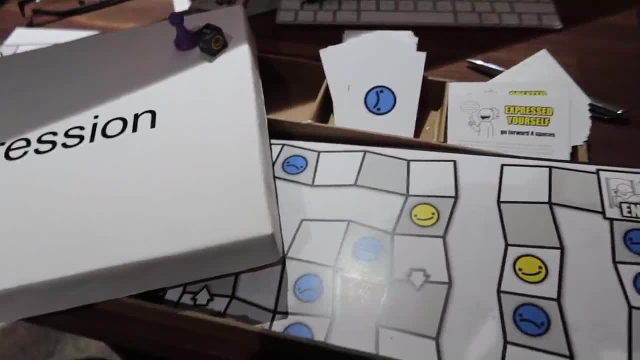 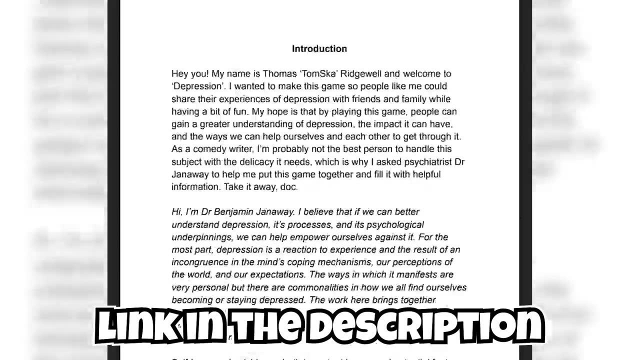 There's a lot I probably won't be able to fit in this video, So I'm also gonna be playing it and talking about it on Dr Jannaway's YouTube channel, which I'll link in the description And also if you wanna download a printable version. 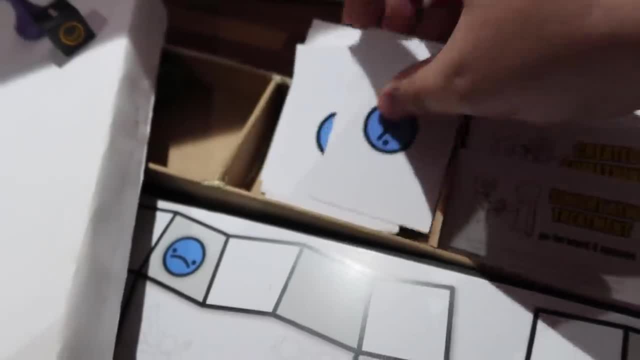 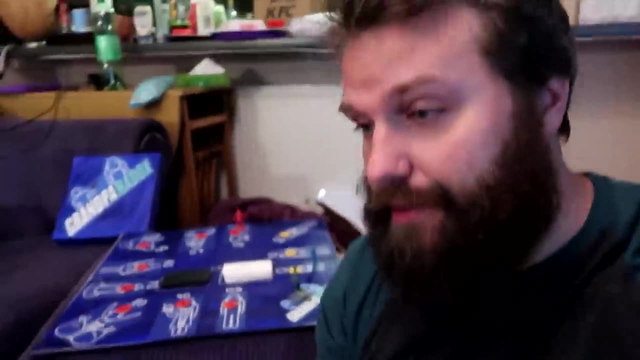 of this game and play it yourself. I'll link that in the description as well. I'm happy with this. Yeah, Yeah, Yeah, And that's it. That's Grand Paradox And I'm really proud of this, And I think this has a lot of potential to the future. 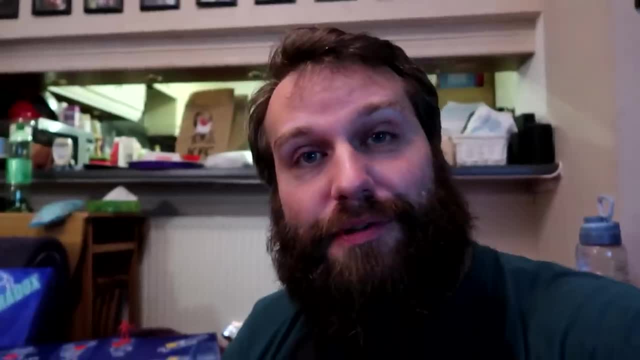 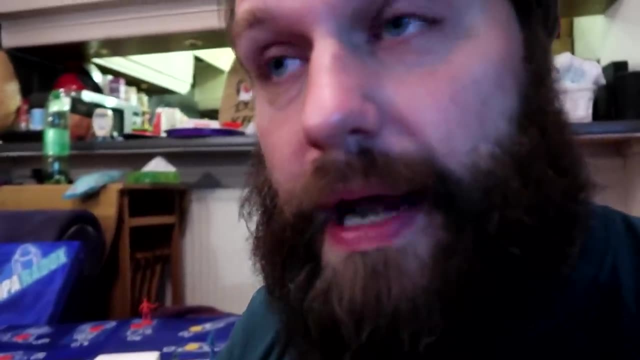 Go to the future. See, we're time traveling to a future, which is what we're always time traveling, If you think about it. we are always time traveling. We are always going forward, never backwards. It will never end, It will never stop, no matter what. 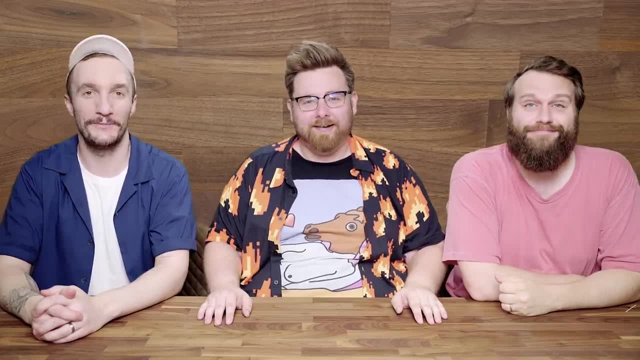 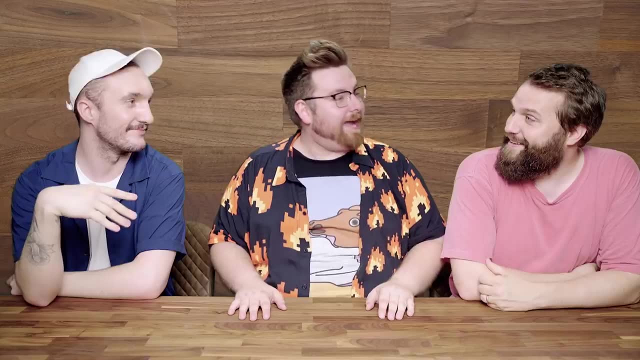 We're in the same room. What? This is so fucking hot. This is the water. It's almost day. Why did we do this? Did you make game? I did make a game, We sure game. Eddie, you go first. 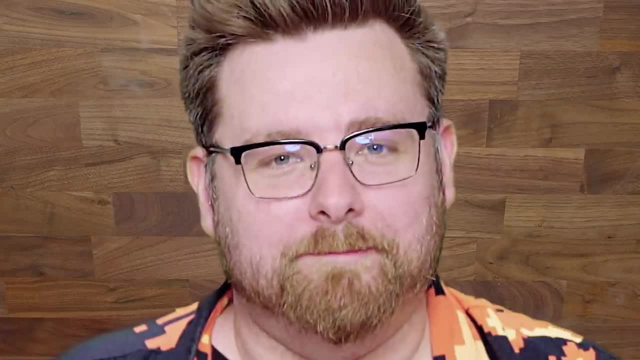 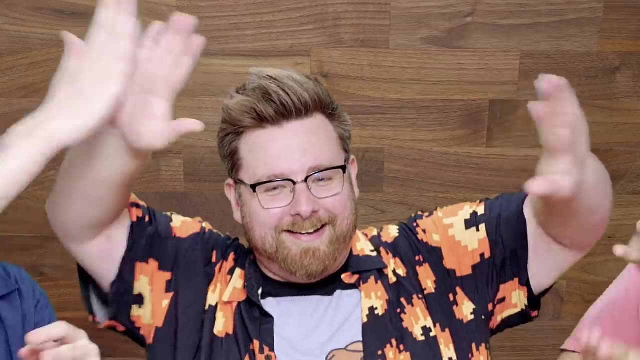 Eddie, you go first. Did you know boys? Nope, Never met one. We all have the same grandad. Is yours dead too? Yeah, Oh, Dead grandad squad. Not only do we all have the same grandad, 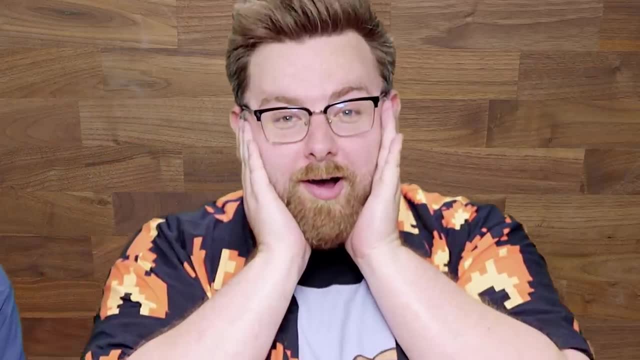 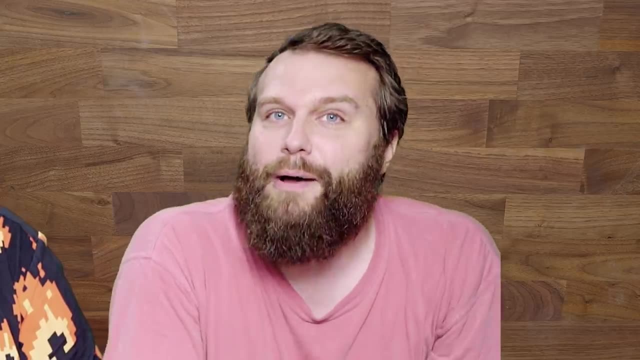 but this grandad has to die. Whoa Mine is dead. Yeah, he's already dead. May I introduce you to Grand Paradox? It's a game about going back in time and killing your own grandfather. Why are we killing him? 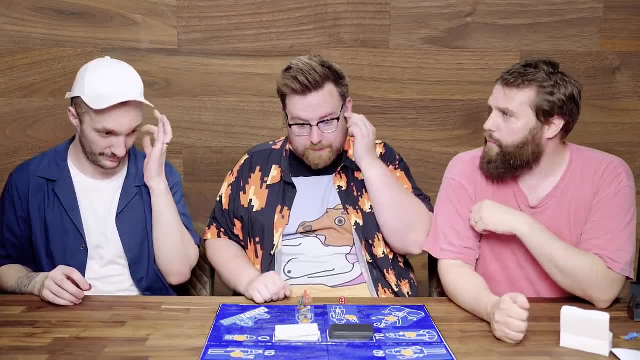 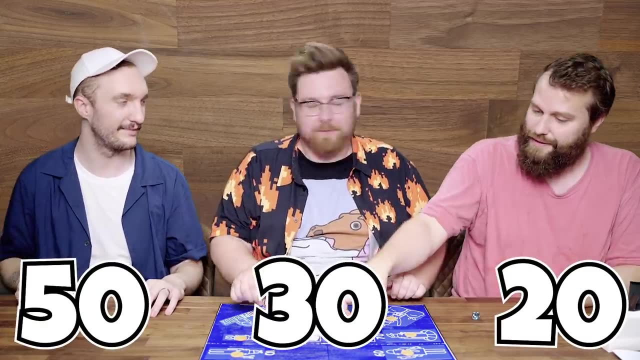 That's a very good question. First of all, we have to figure out how old are. we Go ahead and roll your dice: One spot equals one decade. I am 20.. I'm 50.. I am 30. Okay, 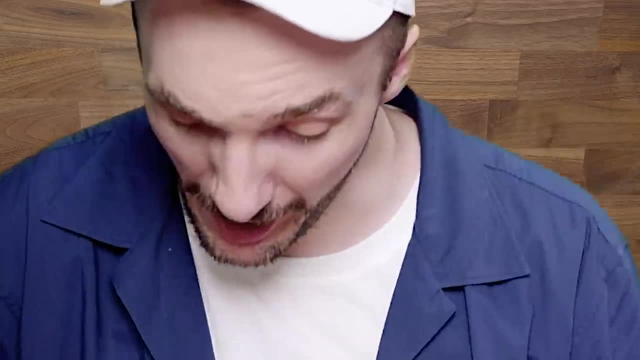 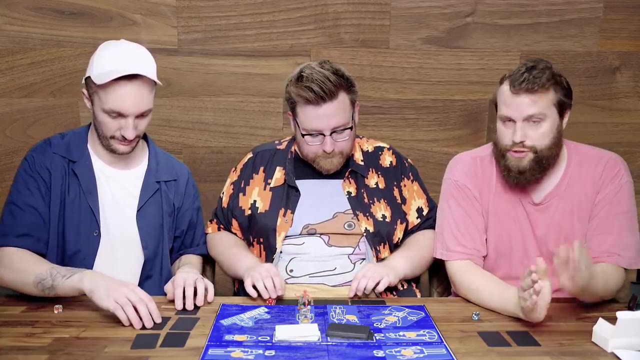 I'm actually 31.. So the older you are, the weaker you are. So No, Die boomer. Let's say we go to kill grandad. It is a mathematical equation to work out. It is your age minus grandad's age, plus your age. 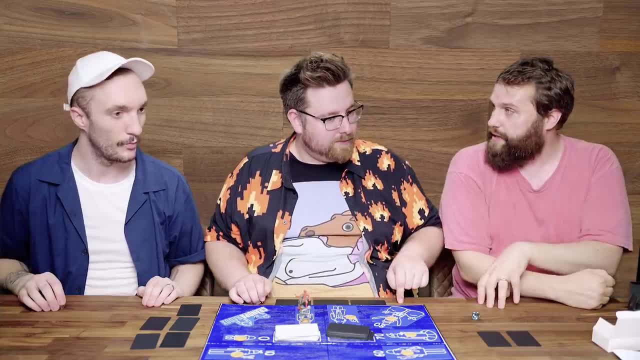 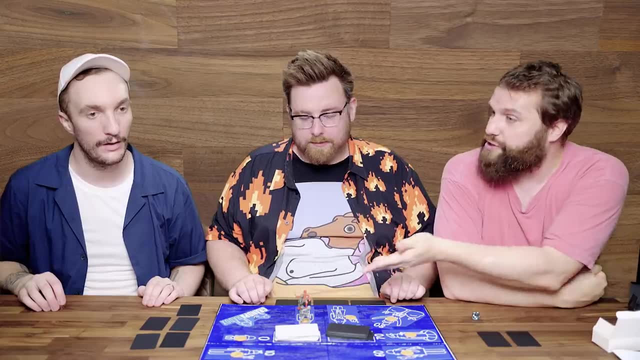 Plus 100, that's the score to beat. You're 30, minus 100, plus 100. So right now you would have to roll a three, four, five or six to kill him. So, 100 years old, he's super weak. 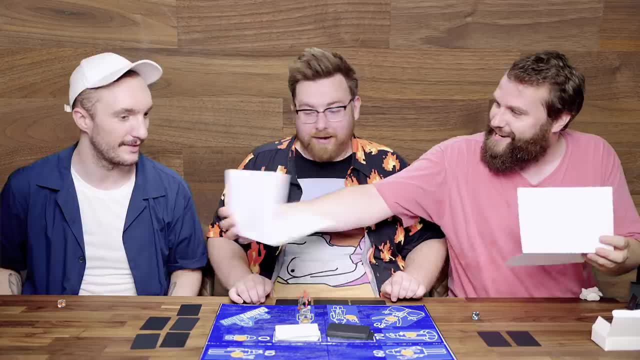 I'll get it. I did prepare these overwhelming flow charts to help you keep track. Oh, this isn't helping. Don't worry, this is a guide. Don't worry, You're not expected to take this all in immediately. That's fucked. 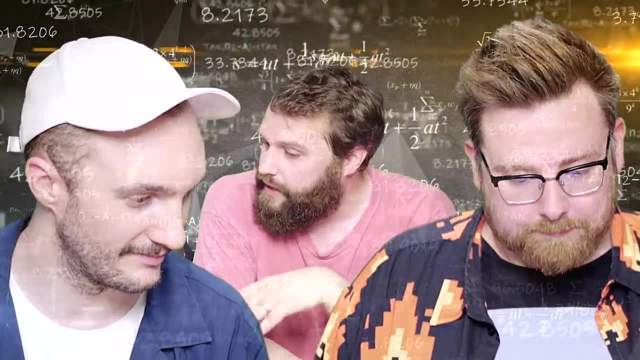 So right, I'm still explaining the rules. Along the way of the game. you collect these weapon cards. If you want to go back in time and kill grandad, you roll the dice Also on your turn if you don't want to kill a grandad. 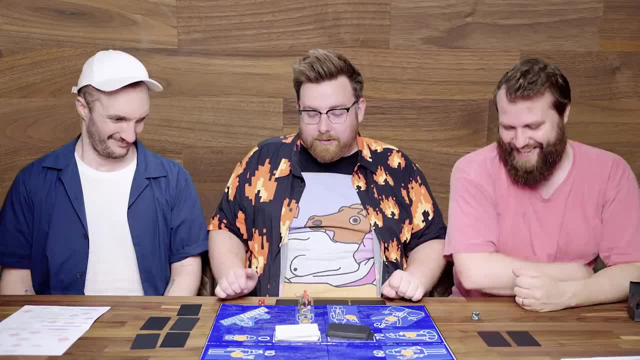 you can collect a weapon. So older grandads are easier to kill than younger grandads. All right, so I'll go first. So I'm going to go ahead and kill this 100-year-old grandad. That's kind of like easy pickings for me. 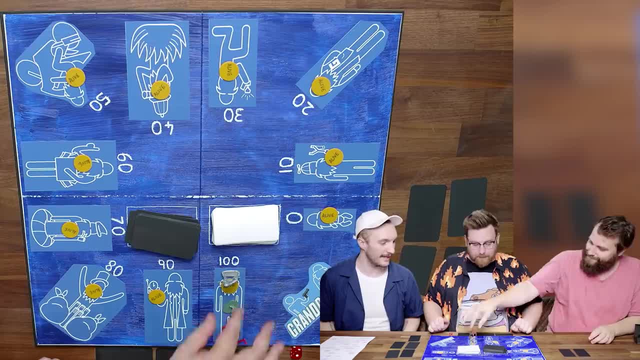 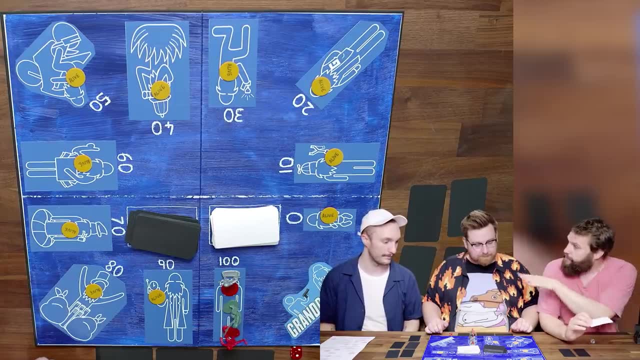 So I'd have to roll a two or above to kill him. I rolled a four. He's dead. So we flip that over. We win For killing grandad. anyone who's in the same space and bat inherits weapons. So I get two, you both get one. 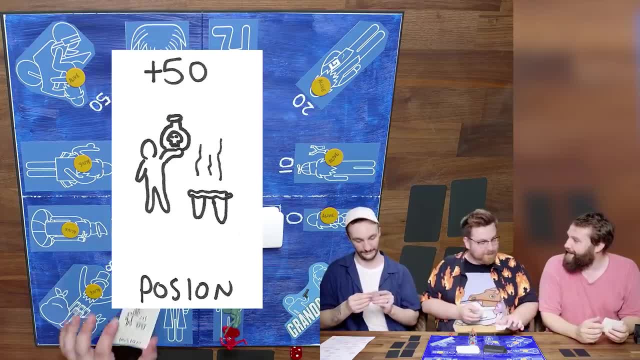 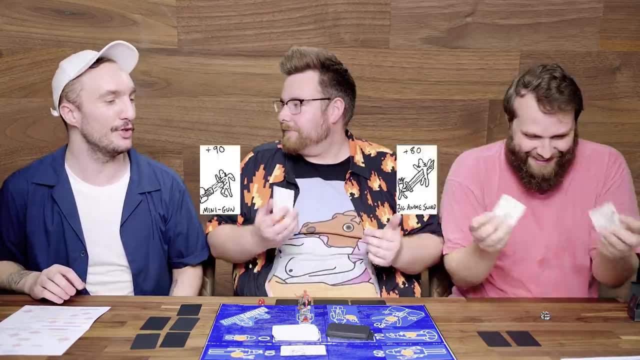 Fucking A. So take a weapon Plus 50 poison. Yeah, what did Elliot get? Nothing. I have a mini gun and a big anime sword. You don't need these things. I feel like he's rigged this. He let us pick up first. 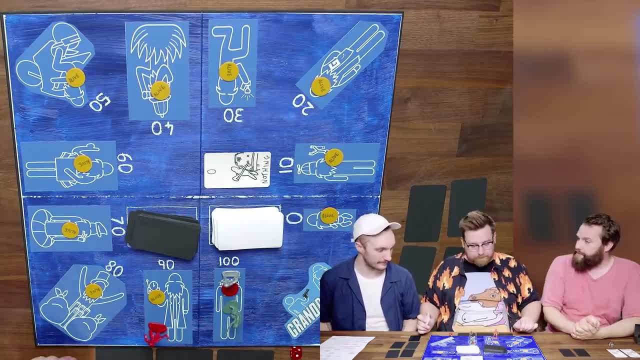 That was fucked up. 90-year-old grandad: your age is 30 minus grandad's age, which is 90. That makes it negative. 60 plus 100 makes it 40. So you'd have to roll a four, five or six to kill him. 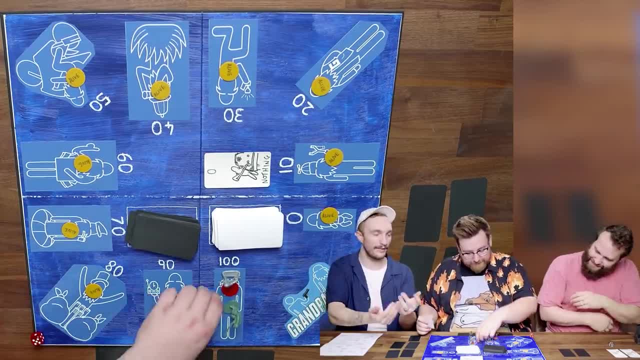 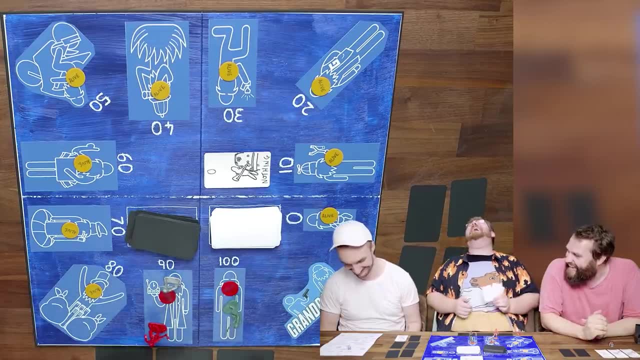 I got a five. Yay, he's dead, Grandad dead. Fuck you, ugly Weapons One. You can't do anything. He's already dead. No, that's on your next turn. You got a six. You got a six everyone. 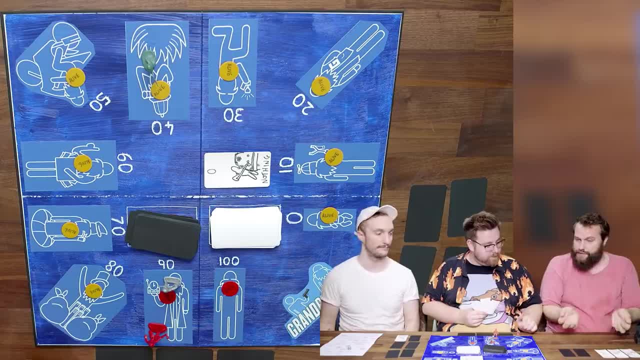 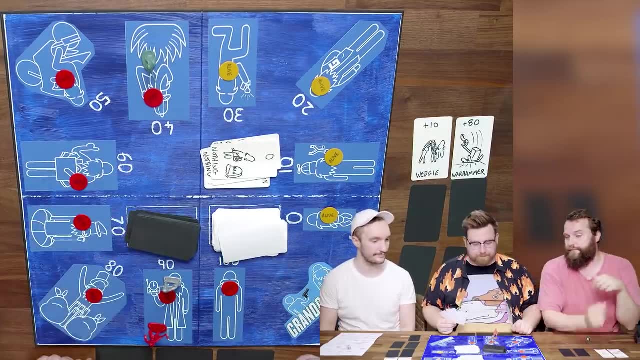 One, two, three, four, five, six. I have a big anime sword, so he's good as dead. All right, he's dead, Yay, Oh So he's dead, dead, dead, dead. If you get a six, you can get a 30-year-old. 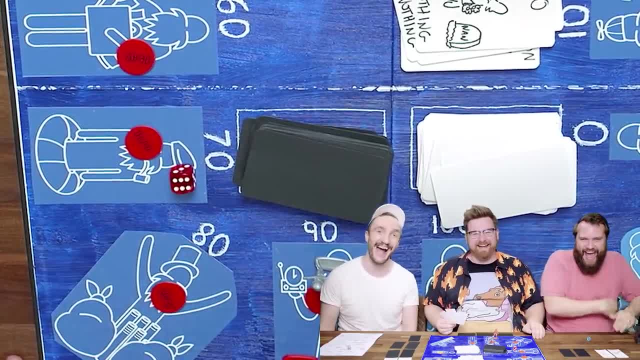 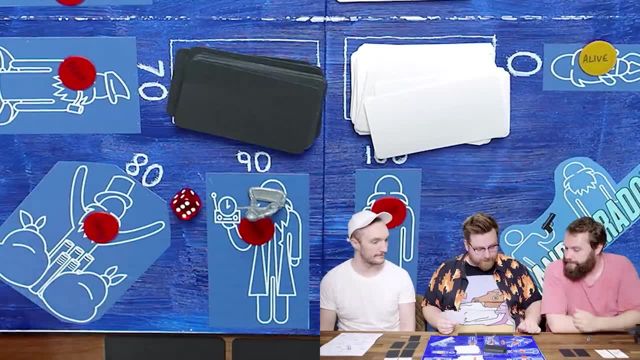 Okay, Wow, What the fuck. I'm very good at games, So you're 30 and he's 30. If you get a five, you can use your 50.. Okay, Stop doing that. Yay, he dead. 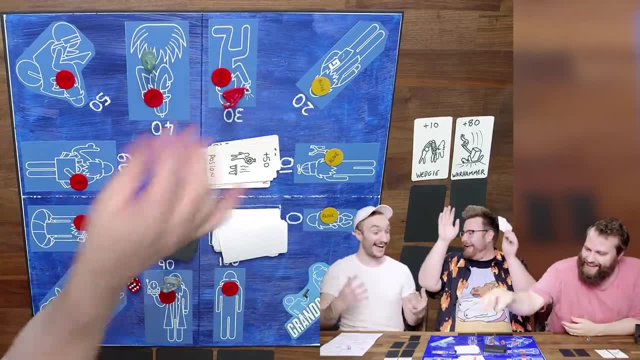 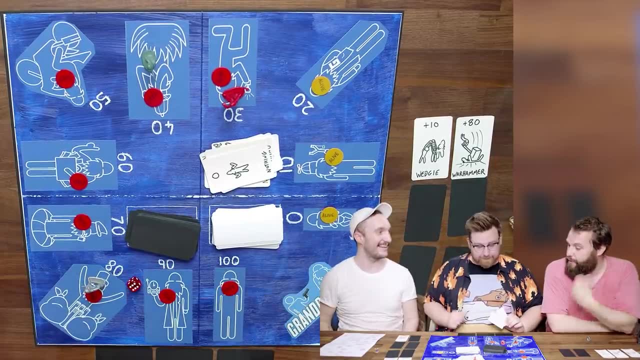 I rolled poison. All right, You use a poison, He's dead. Weapons, Weapons, Elliot, that's a one, Yay One. You've gone back in time. I mean It is time. Can he do nothing? 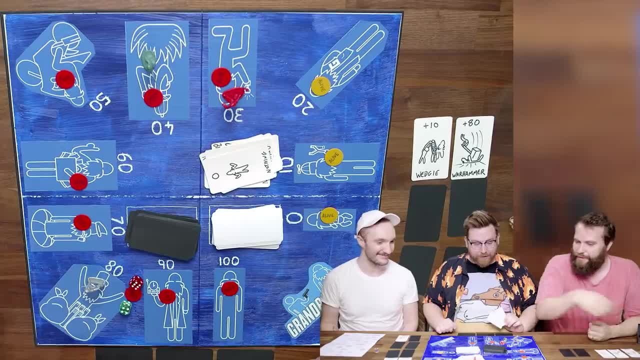 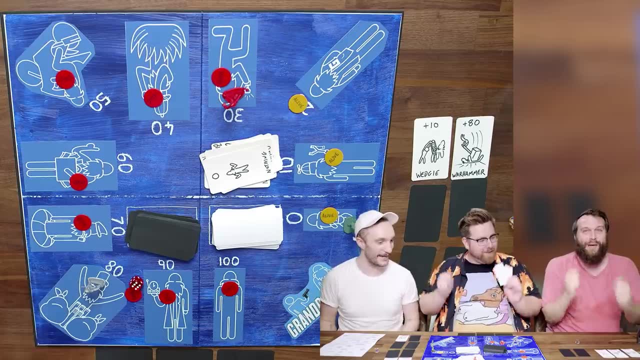 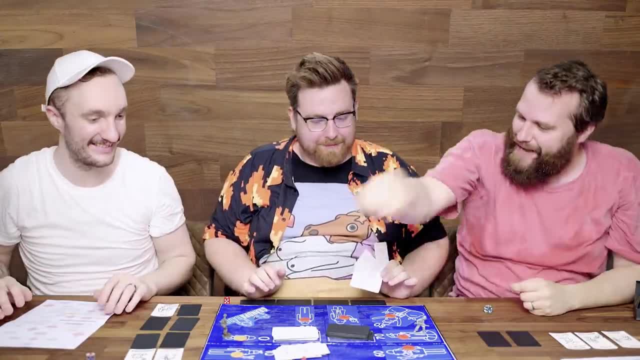 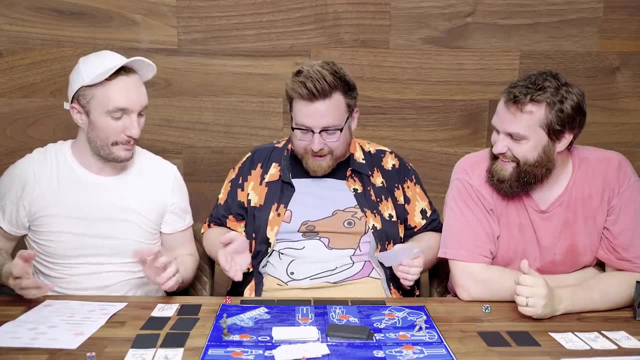 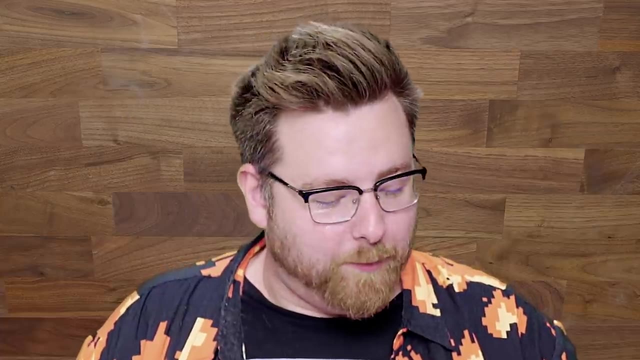 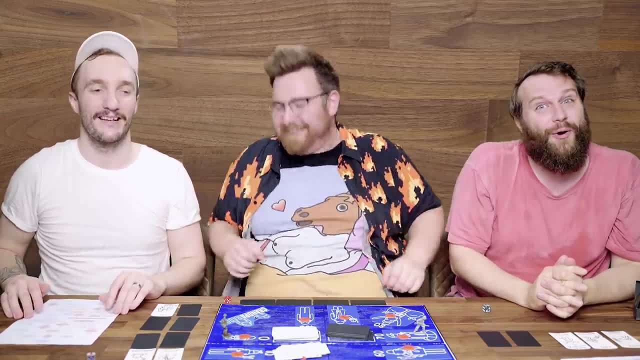 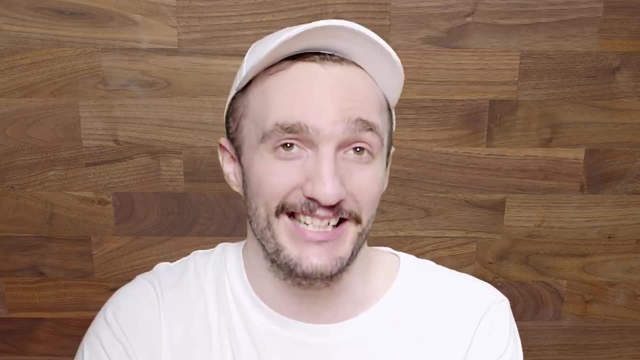 We're going to turn some fans on by getting undressed Elliot. I'm going now, I guess. So have you guys ever played the Pokemon trading card game? No, No, God, it's complicated. What if I made it a very simple party card game? 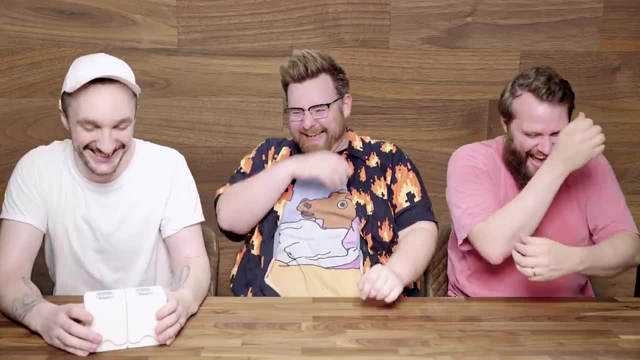 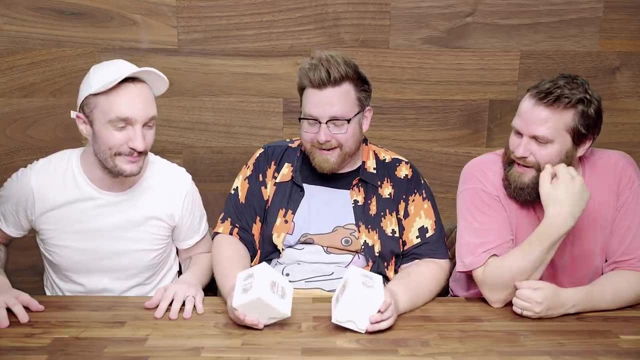 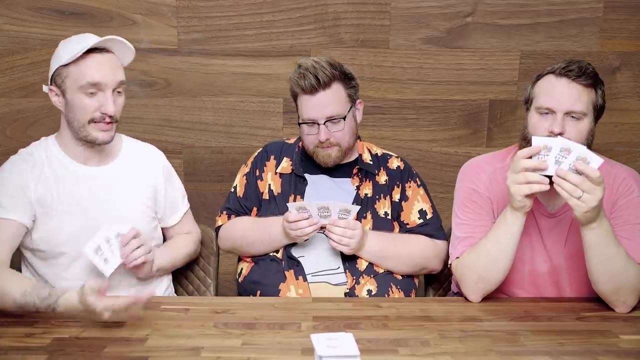 So welcome to It's Pokemon Time. What is this, Elliot? this is Pokemon. It's Pokemon Time. You're breaching two copyrights, Elliot. I made this myself. Essentially, you've got to pick a Pokemon and we see who wins. 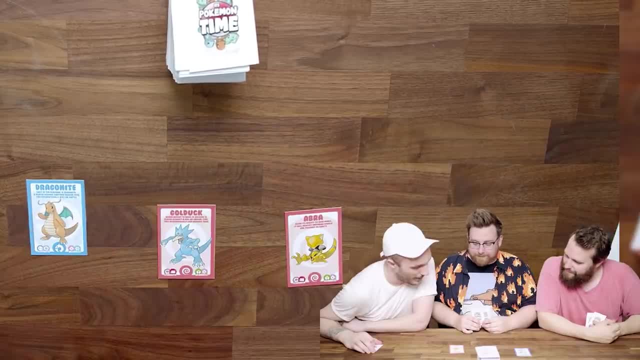 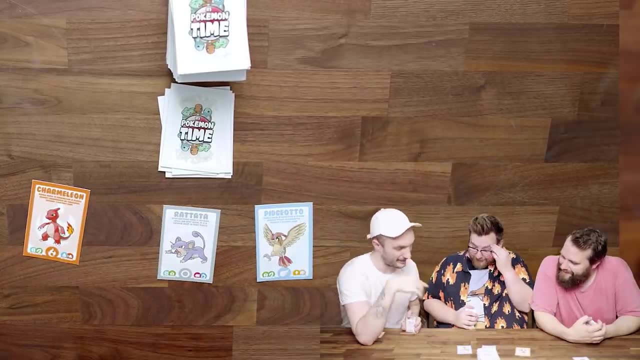 So let's go for it: Three, two, one, Nobody wins, Yay. And then they all just go: three, two, one, Ratatouille, Ratatouille, million, And no one, Nope, Nobody wins. 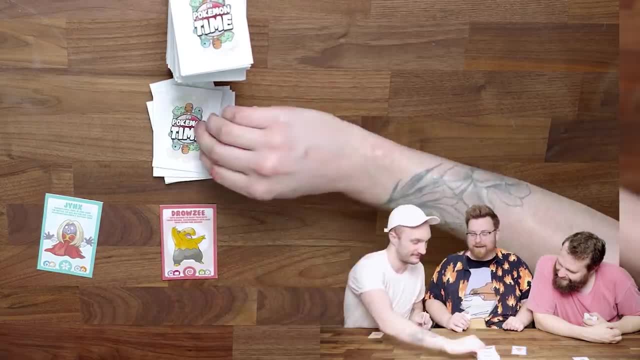 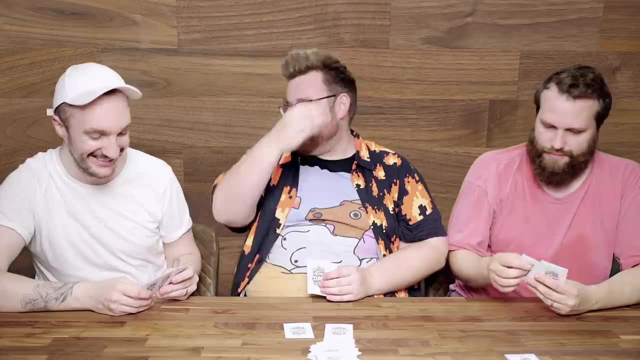 Yay, I did nothing. Nope, Nobody wins, Nobody wins. I didn't expect so many no wins. God damn it. Nobody ever. Yeah, this feels good. All right, Let's rebalance it. so now you get a victory card. 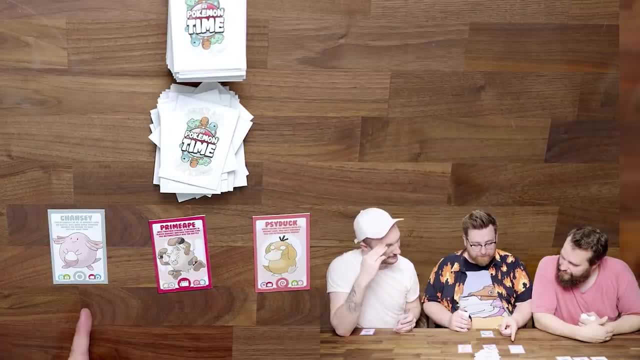 even if you knock out one person, Three, two, one- So I knocked you out, but he knocks me out. But if I lose, I play rock paper scissor against the winner and take the victory from them. Oh my god. 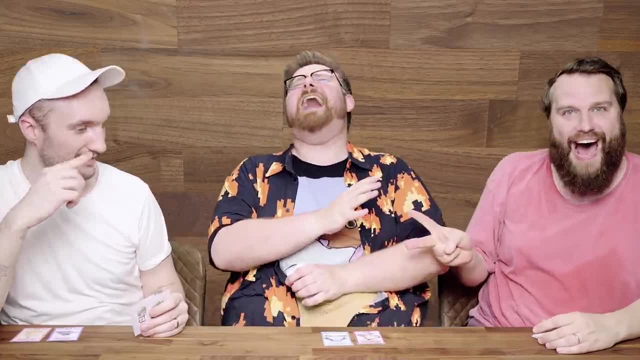 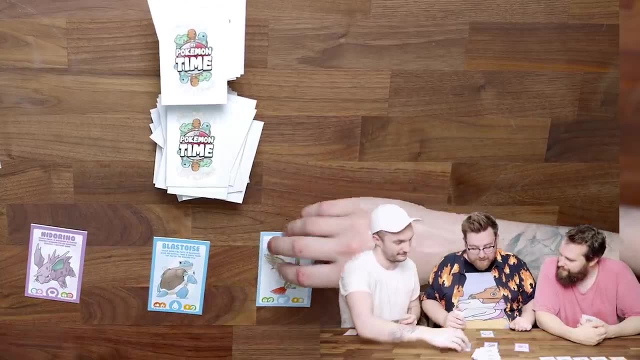 OK, So I have to play rock paper scissors. go, Ha ha Ha ha. OK, Uh, I'm going to shit. Oh, nobody wins. Nobody wins. Three, two, one, Go, Reveal, I'm strong against nothing. 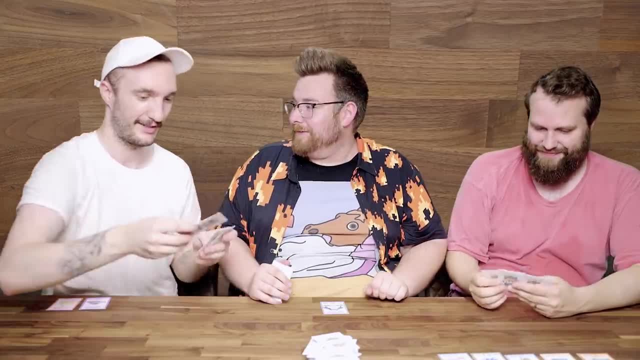 God fuck, God fuck. Would you like to stop? It's a great game. Would you like to stop? This is great. I'm enjoying it. He's winning. He would enjoy it. Three, two, one Go. 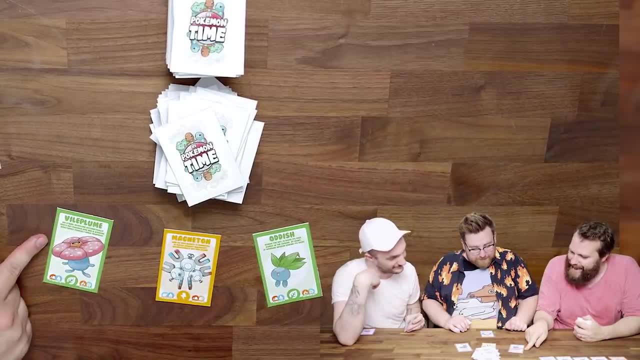 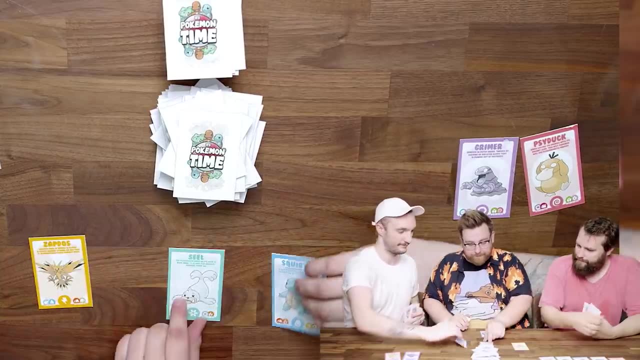 Magneton Strong against Fuck. Oh, Oh, I'm good against any Pokemon that has a nose. Ha ha ha. Nice dude, Not one of you have a fucking nose. Three, two, one Pokemon, Yes, OK. 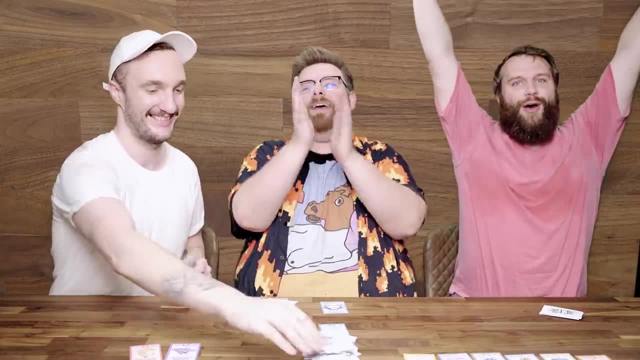 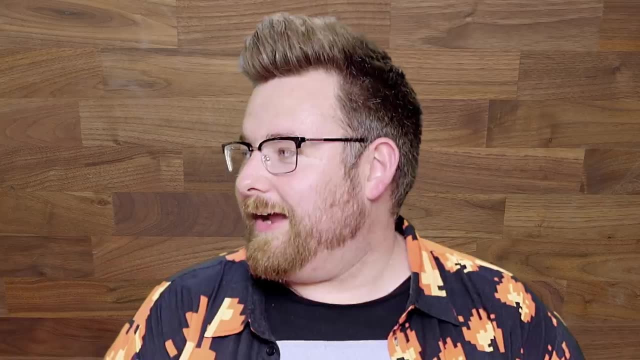 Who wins against me? Oh my god, Yes, Eddie wins, Eddie wins. Woo, Woo, Woo, Yay, Yay, Yay Yay. I failed to make Pokemon better. Ha ha ha. Elliot, Tom Elliot, how are you feeling right now? 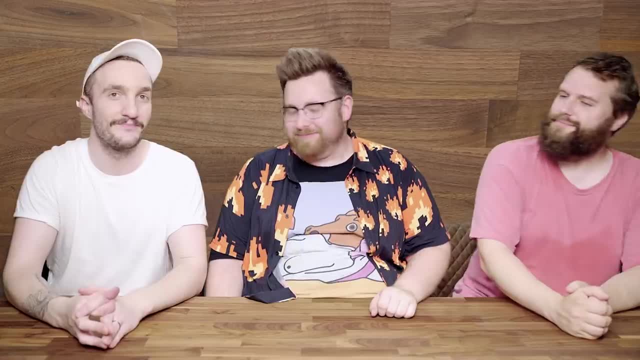 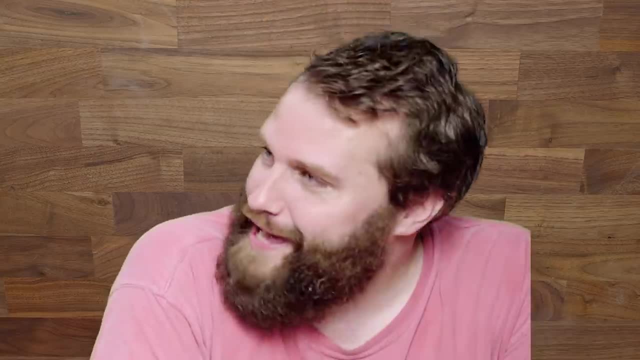 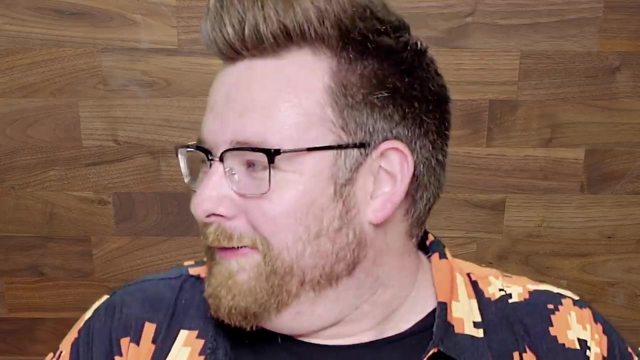 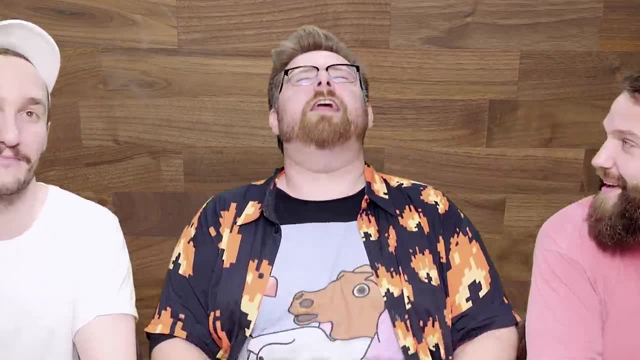 I definitely didn't see this by accident in your emails, Tom. No, Ha ha ha. So this is depression. The rules of the game are: you start your day and you gotta just guess the end of your day. Just get through your day. 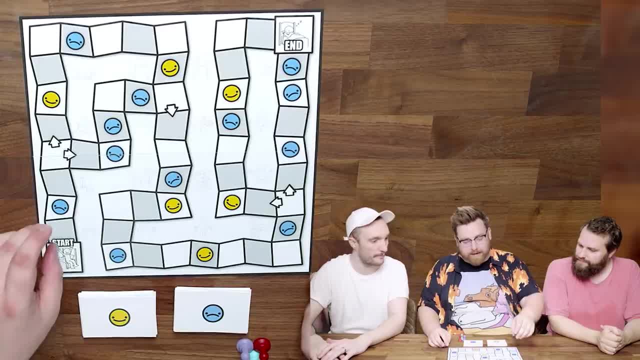 So you roll the dice: You'll either get to move forward one, two, three or four, or you'll land on a sad face or a happy face. Then draw one of those cards and you'll find out what it does. 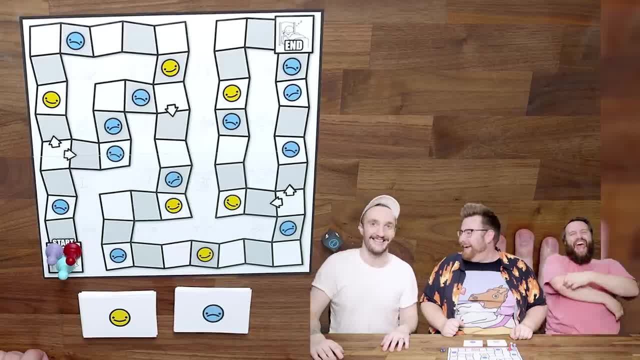 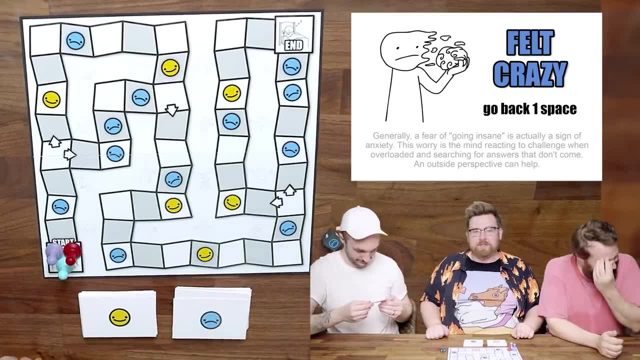 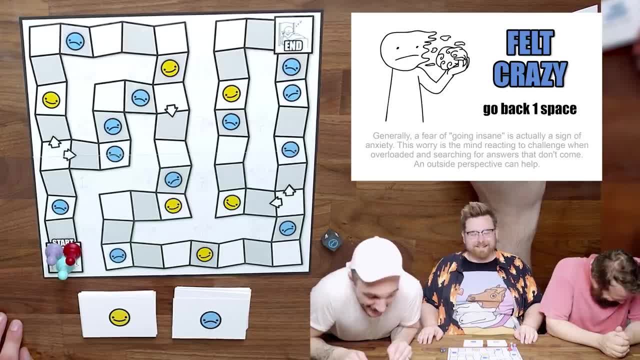 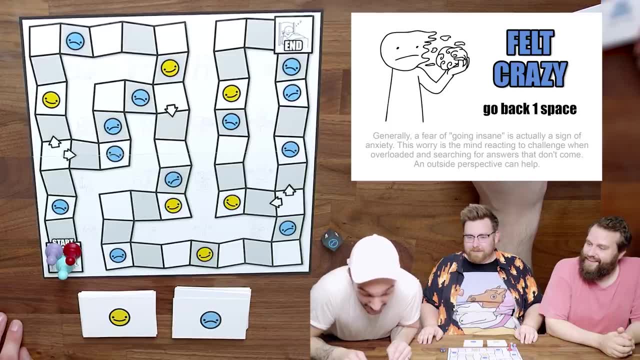 Generally, a fear of going insane is actually a sign of anxiety. This worry is the mind reacting to a challenge when overloaded and searching for answers that don't come. An outside perspective can help, Like talking therapies. Go on, do it again. 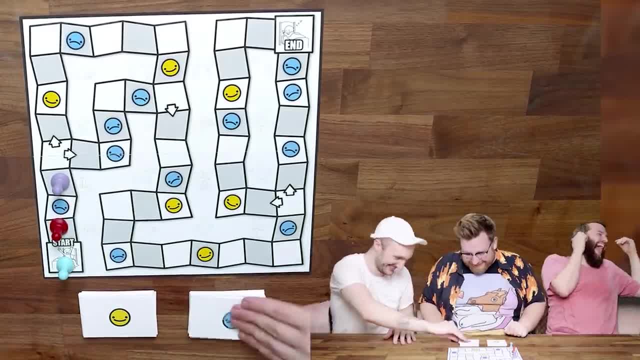 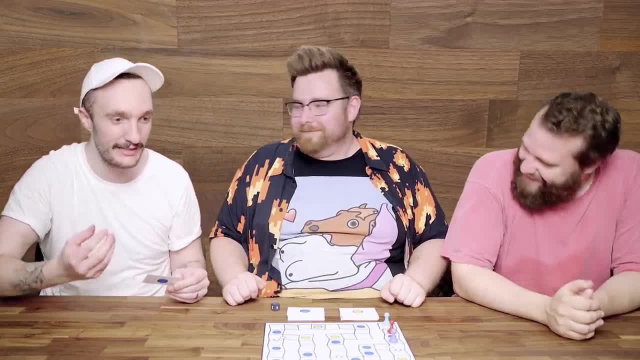 Do it again. Ha ha ha, Ha ha ha. Depression, Depression Got angry, Ha ha ha. Depression can lead to anger. Depression And anger can lead to fear. Ha ha ha, And anger can lead to the dark side. 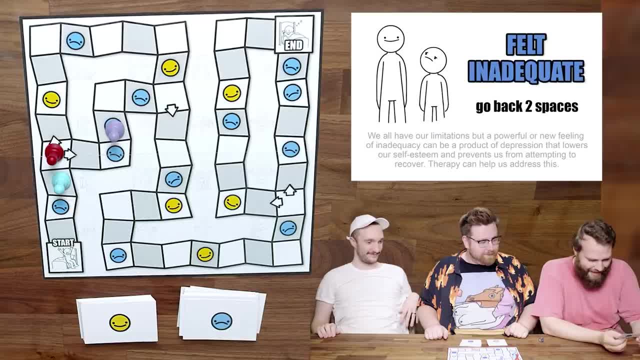 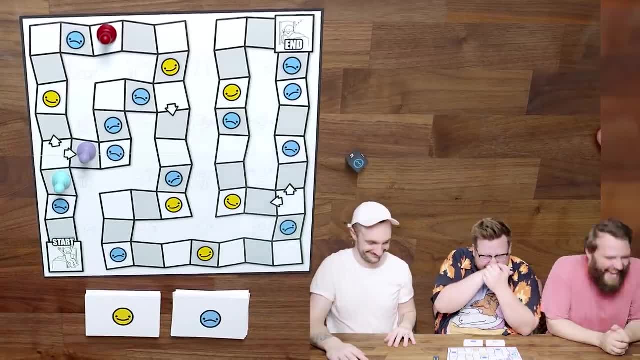 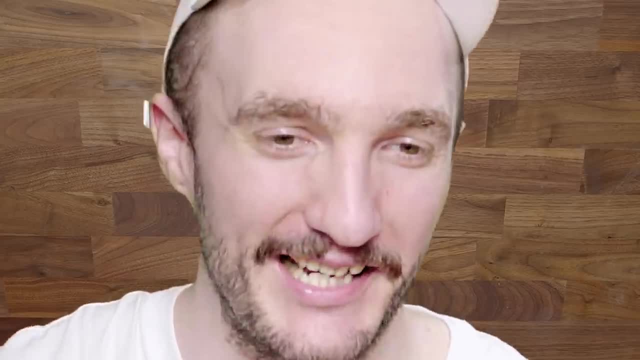 Ha ha ha. That's not what it says. Go back two squares. Why? Why? Because I felt inadequate. Good, Listen to those demons. I'm so fucking sorry. Avoided recovery. Go back five squares. The gods have forsaken me. 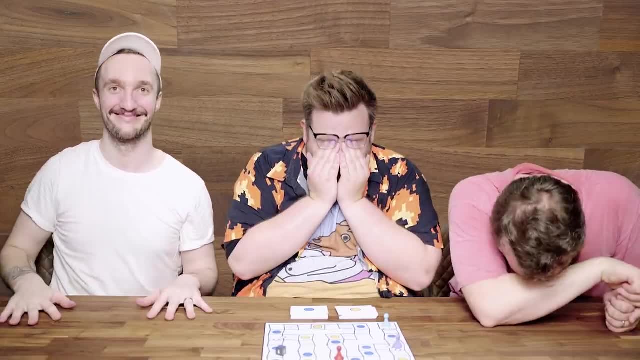 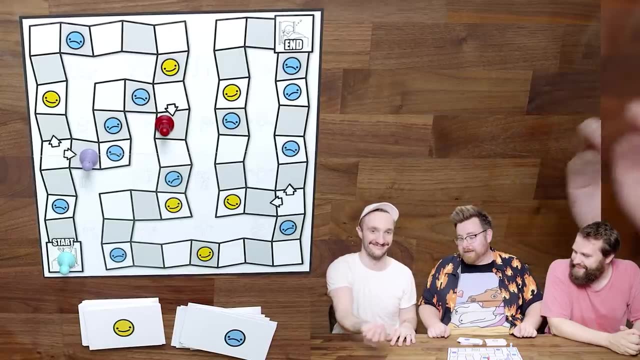 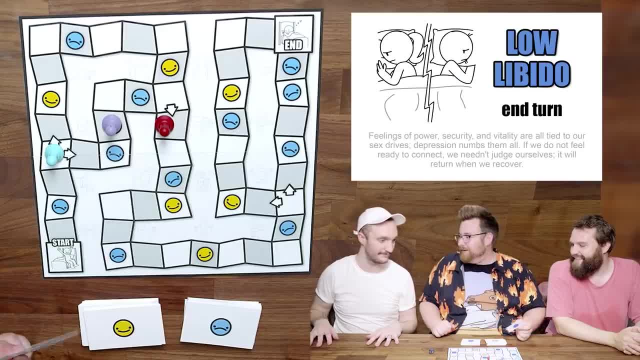 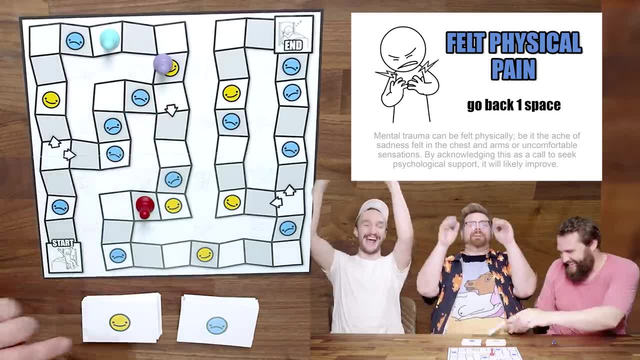 Ha, ha ha. Yay, Oh, I lost my sex drive. Beep, beep. Sorry, honey, I felt physical pain. Go back one square, But I'm happy again. Yay, You found an unhealthy coping mechanism. I won't lie. 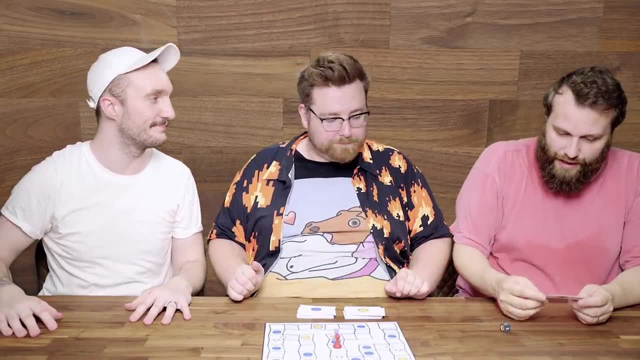 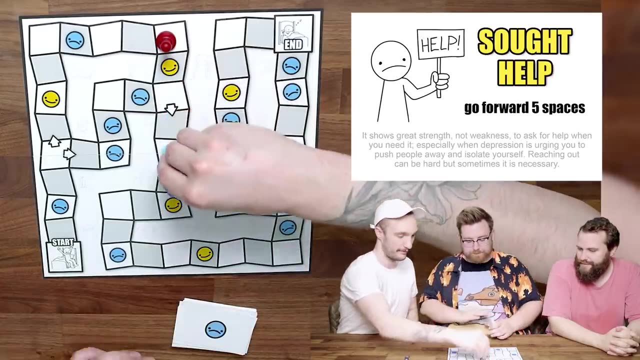 I may have balanced this a bit brutally. Well, at least something's happening. Tom End turn. I stayed in bed. I'm just staying in bed. I sought help Go forward five spaces. Wow, Hey, One, two, three, four, five. 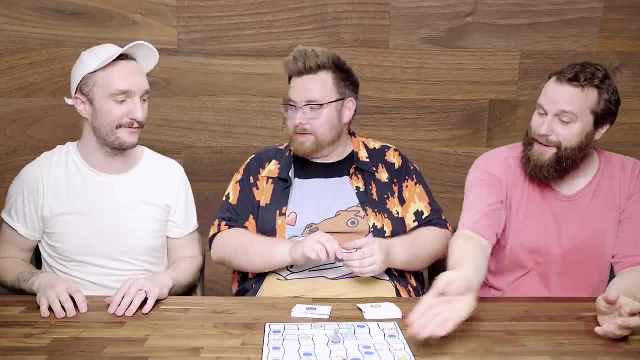 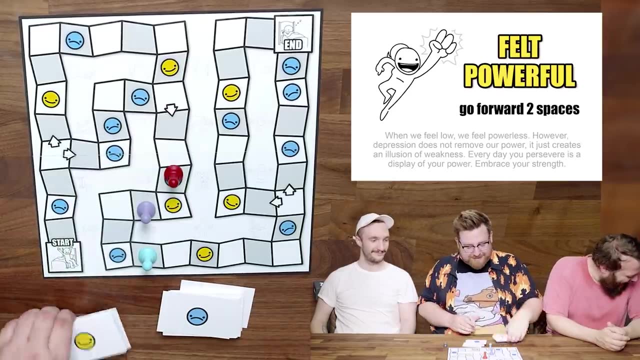 Oh my god, It's the happy time You got help. Wes Come a long way Since being stuck in bed. You really have I felt powerful. I go forward two spaces and I immediately pay for it. Ha ha ha. 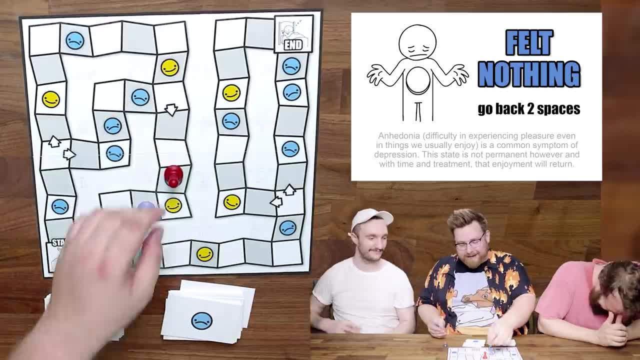 You're hubris, My hubries. Oh, I felt nothing And I go back two spaces. I felt powerful. It was a fleeting feeling. I wanted to run away, Go back one space, But then I got happy, because I fucking hate my family. 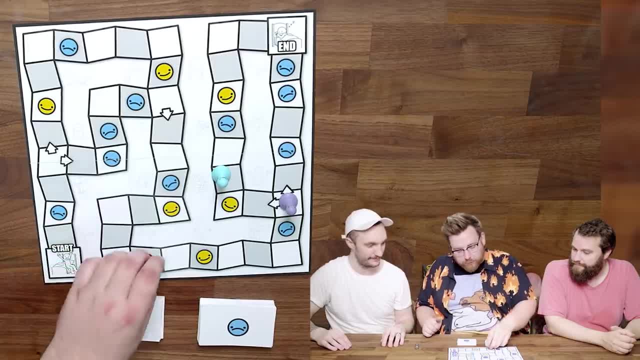 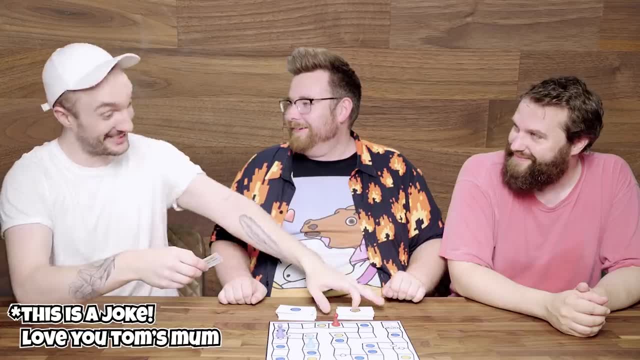 Ha, ha ha. Oh, what the fuck? Four. One, two, three, four. Da-na-na-na-na-na-na-na-na Explored- Go forward two spaces. What did you explore? One, two, Three, four. 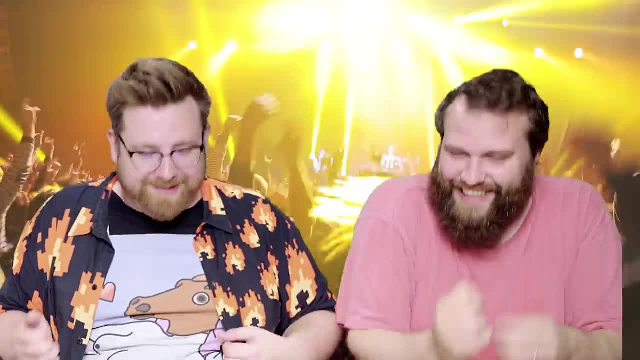 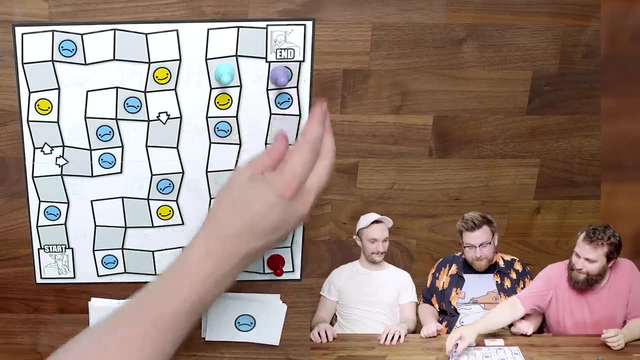 Ha, ha ha, Four. One, two, three, four. Da-na-na-na-na-na-na-na-na Good joke. I'll show you if I do it, again. One, two, three, four. Oh, One, two, three, four. 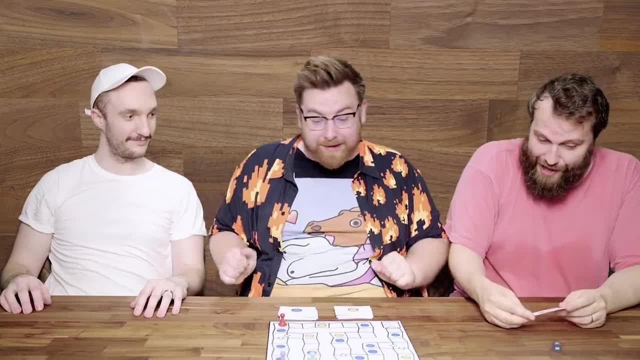 Da-na-na-na-na-na-na-na. Oh my god, If you just get an N-turn, you might be alright. N-turn, Oh, fuck it. Confidate, Confidate. Oh, Oh my god, This is horrible. 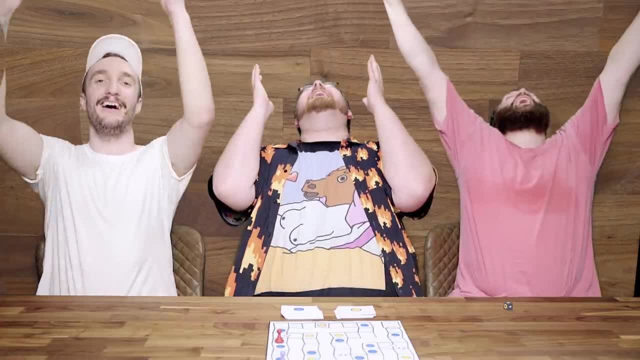 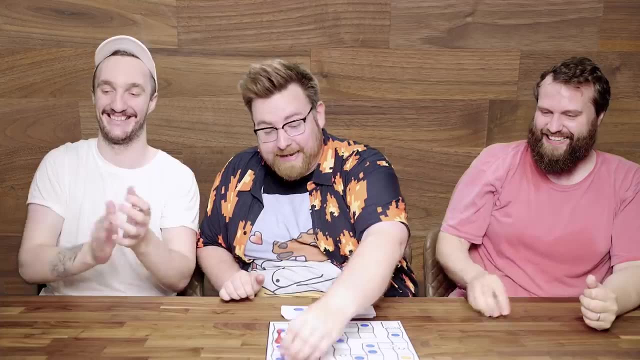 Oh fuck, Come on, Don't you dare, Don't you dare. No, I'm happy. And the moral of the story is: the neurotypicals win. Neurotypicals win. Don't have mental illness. He won every game. 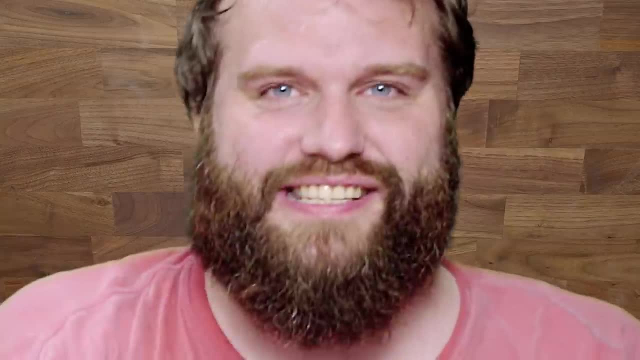 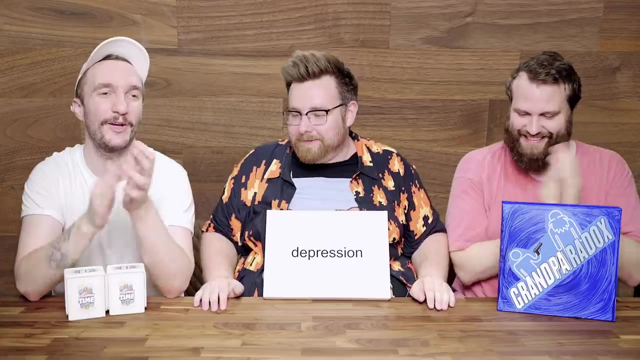 He won every game. I hate him. Yes, I do feel depressed now. Oh, Yay, Yay. We all tried hard, We did Sure did Blah, blah, blah. We have a Patreon. Patreon exclusive podcast. 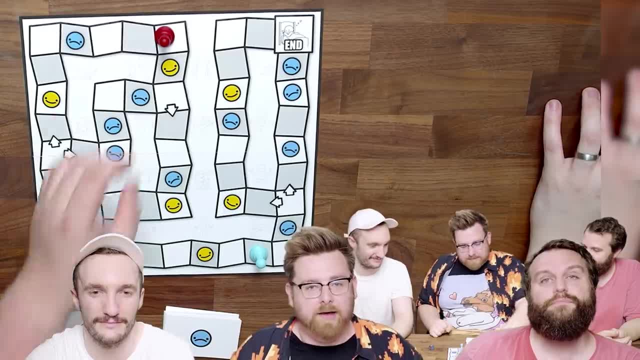 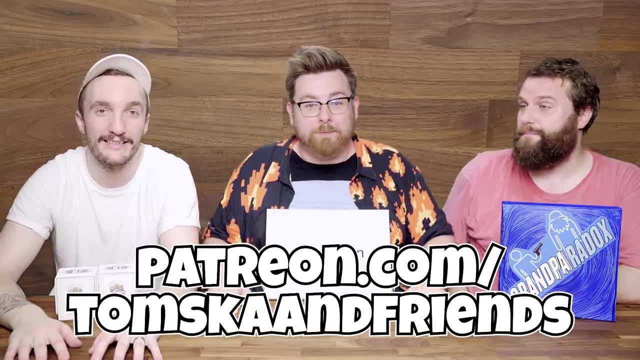 Discord server Extra thing if you want to watch the entire play of us fucking around with these games and getting obscenely sweaty. It smells in here. It smells in here, Panky, You can make another one. You can pay money for that. 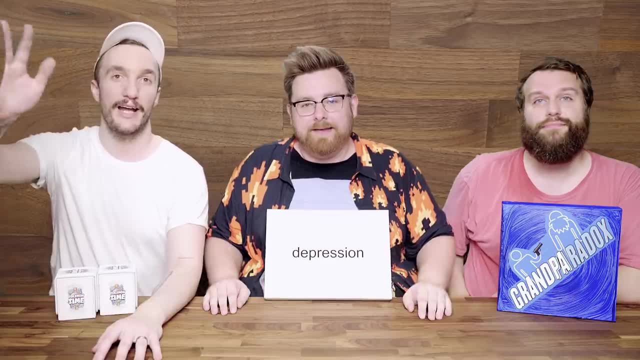 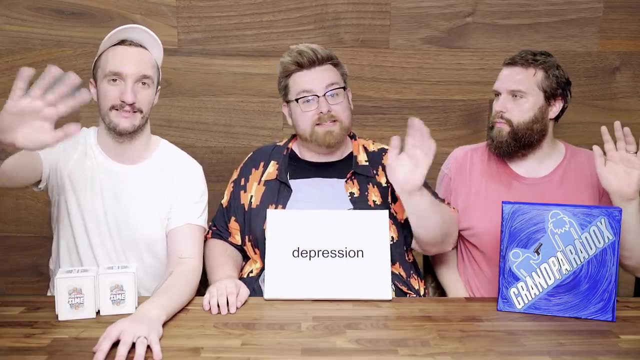 Yeah, It gives a pickboy smell. yes, Yeah, It is musky. Goodbye, Tre DetFC. Good try, Good try, Good try. See you for the series finale, Season finale. Season finale, Not series. 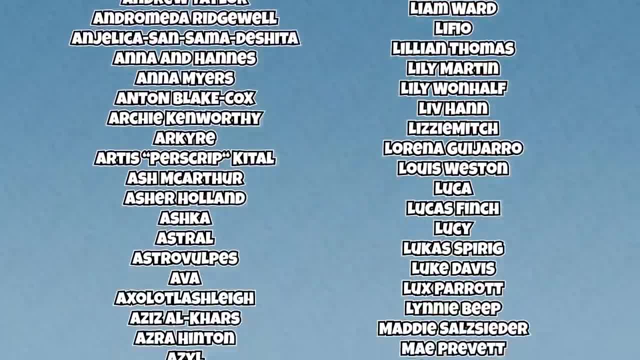 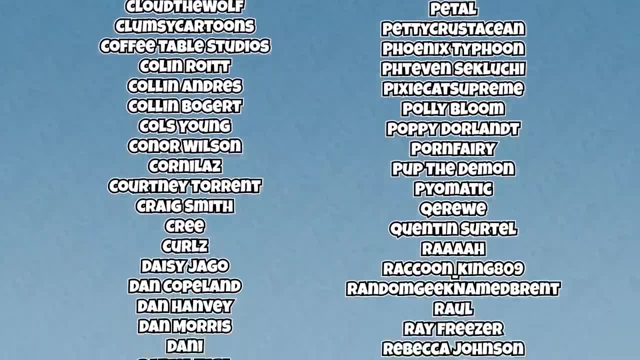 Season finale. What Good-bye? Hey you, Thank you for the money. Hey you, Thank you for the money. Hey you, Thank you for the money Money. Hey you, Thank you for the money Money. Thank you for the money.